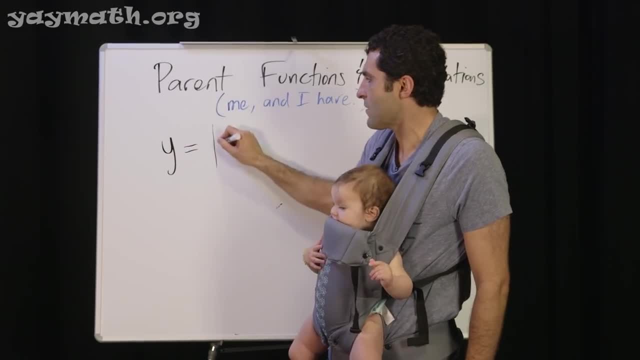 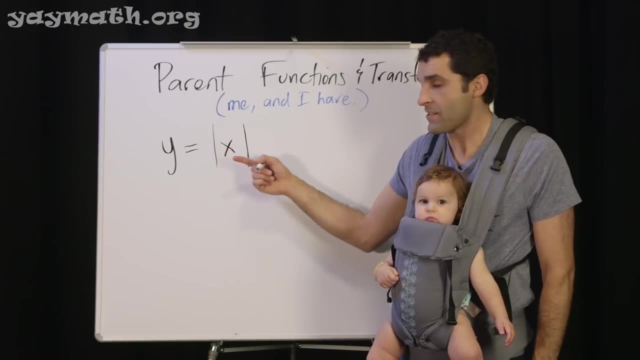 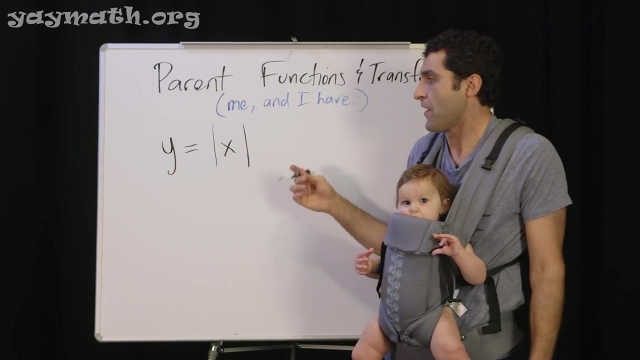 at the board. So let's say we had one function called the absolute value of x. That's one type of parent function. What we can do to this is first understand how it looks, and then we'll start to transform it. So that's what we mean by parent function. It's the original graph. 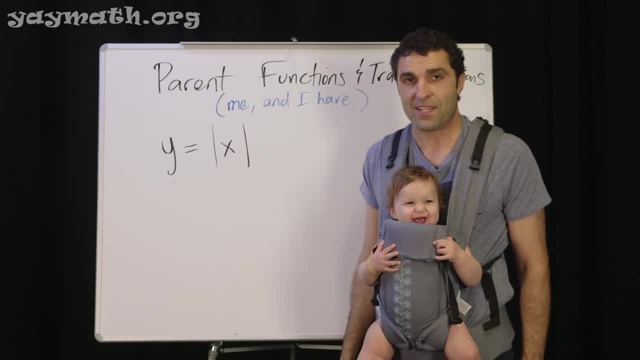 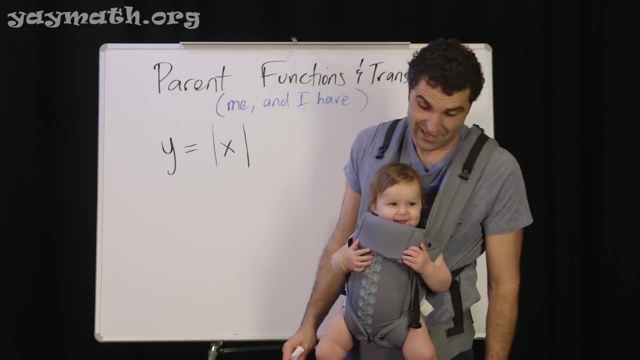 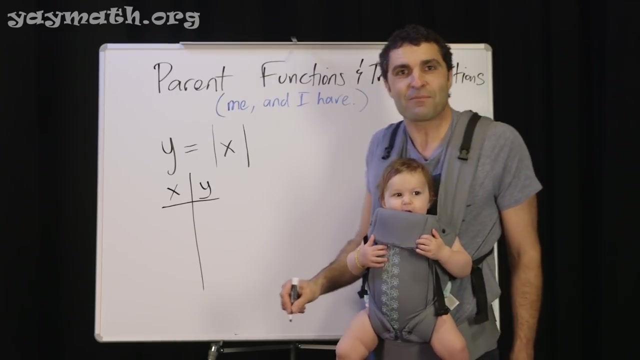 and then what we do to it, to transform it, to make it look like something else. Yeah, transforming graphs is very funny, and transforming my life is actually occurring right now in real time. So let's just do this. So we have either you're happy or something's coming out of your body. 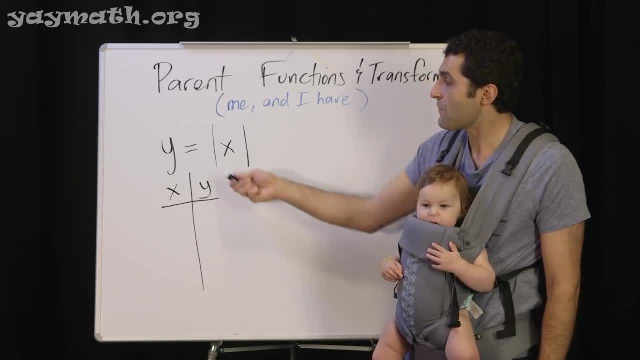 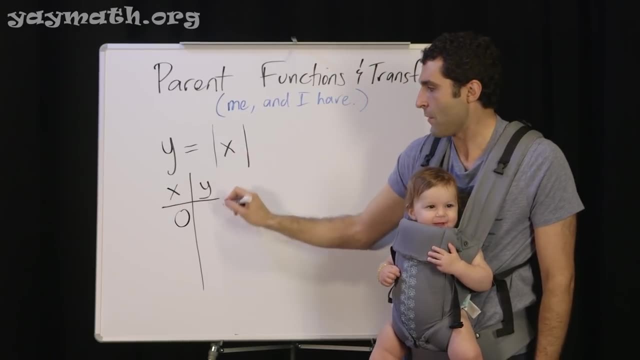 So let's- I hope it's the first- Let's figure out what x and y are. in this case, The easiest thing to plug in is: x is 0, and so if we did the absolute value of 0, y would result in. 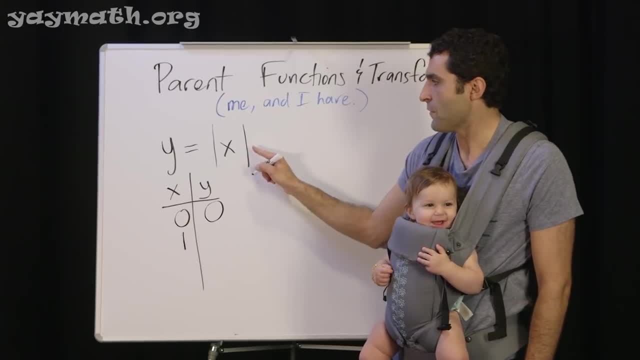 0 as well. We can try 1,. the absolute value of 1 for x is 1.. We could try 2, the absolute value of 2 is 2.. And then we could try a few negative values like x and 1.. And they're actually relatively. 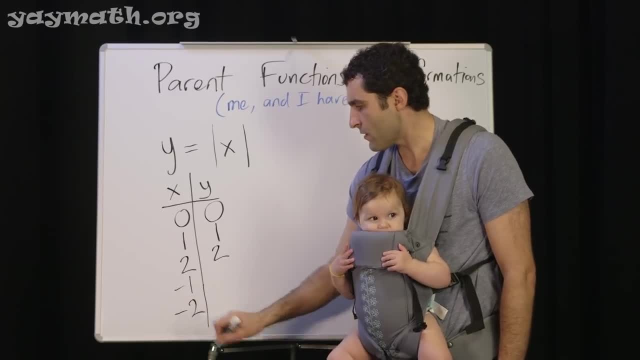 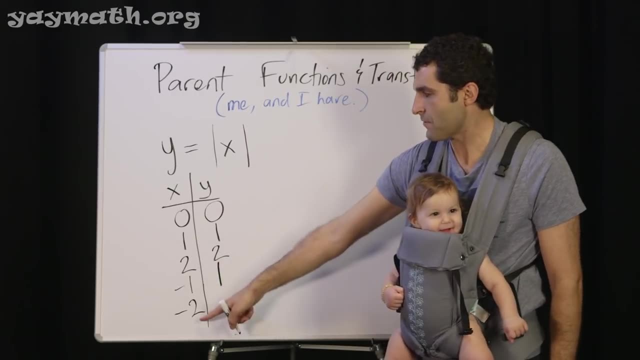 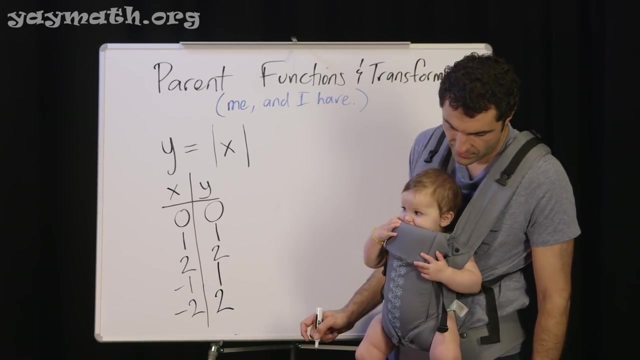 negatives like negative 1 and negative 2? There you go. What is the absolute value of negative 1? if we were to put negative 1 in here, It would be 1.. And the absolute value of negative 2 would be 2.. That's right. Yeah, you want to keep going, Are you understanding? 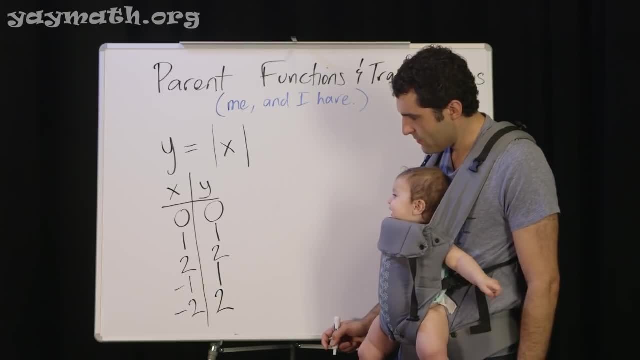 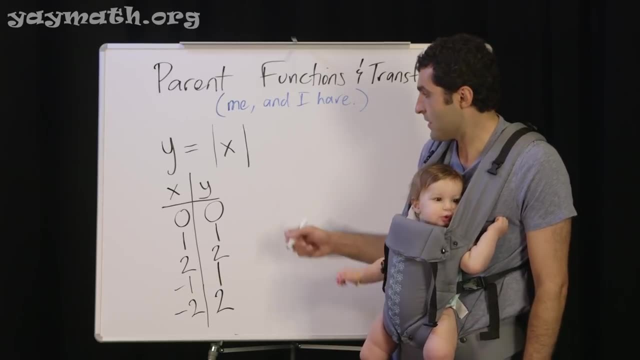 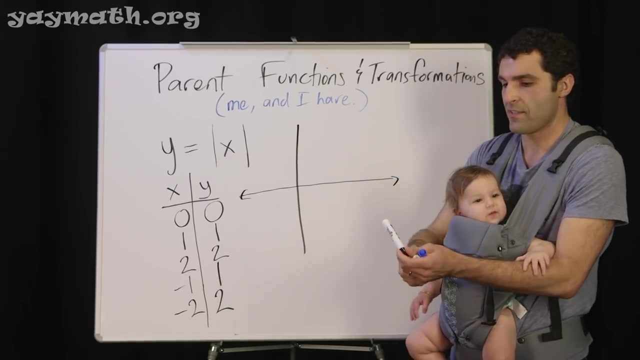 it so far. I find it just as appealing as you do. I really do, But you know what It's going to get- even more insane. Let's do this. Yeah, take a good stretch, because you're going to need it. Here it comes. Let's plot those points. Oh, thank you, This feels so nice. 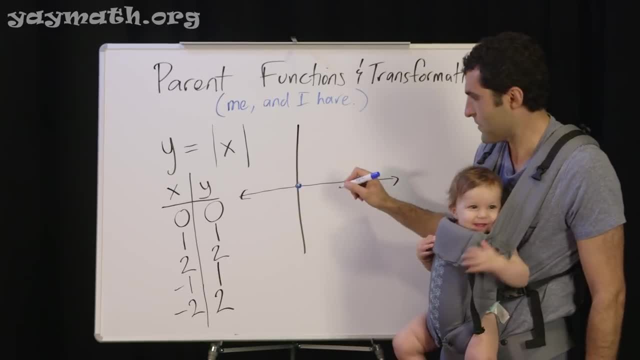 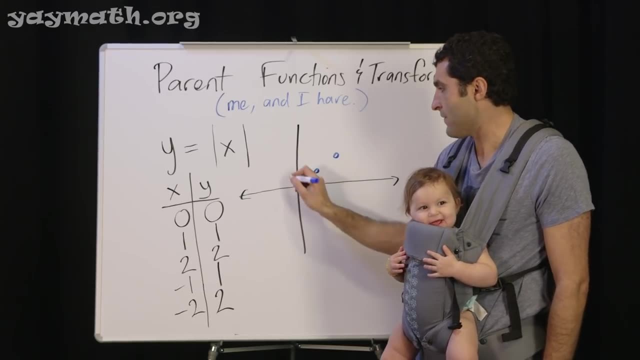 Your skin is insanely soft. I don't know how you do it. Do you use product or something? I'm going to put in 0, 0, 1, 1, 2, 2.. And then you have negative 1, 1 and negative 2, 2.. 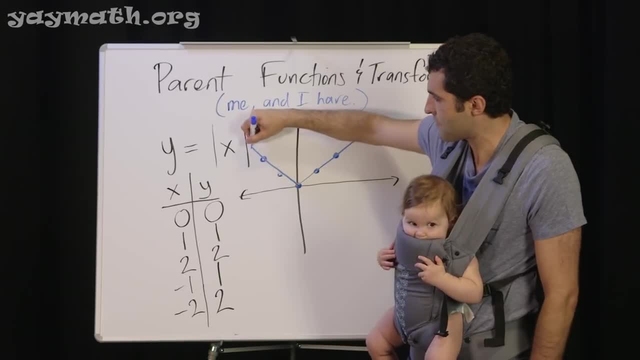 Absolute value looks like a V, And the way I remember it with my students is I'm going to put in 0, 0, 1, 1, 2, 2.. And then you have negative 1, 1 and. negative 2, 2.. And then you have negative 1, 1 and negative 2, 2.. And then you have negative 1, 1, 1,, 2, 2.. And then you have negative 1, 1, 1, 1, 2.. And then you have negative. 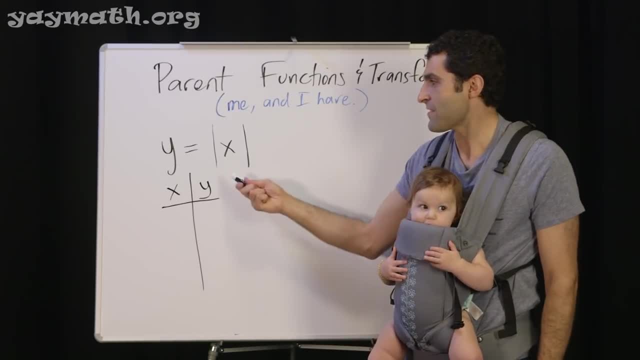 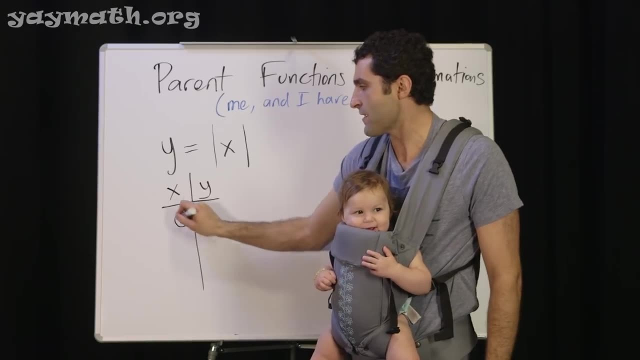 you're happy or something's coming out of your body. So let's- I hope it's the first- Let's figure out what x and y are. in this case, The easiest thing to plug in is: x is zero, And so if we did that, absolute value of zero, y would result in zero as well. We. 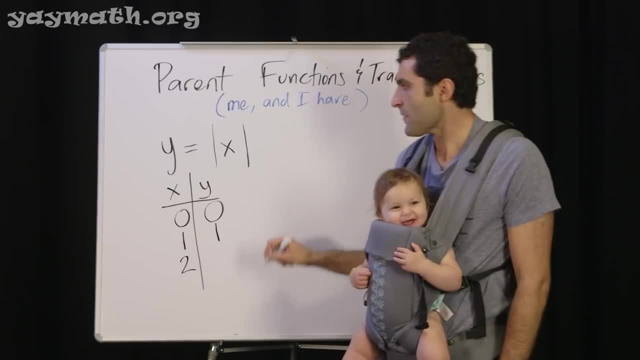 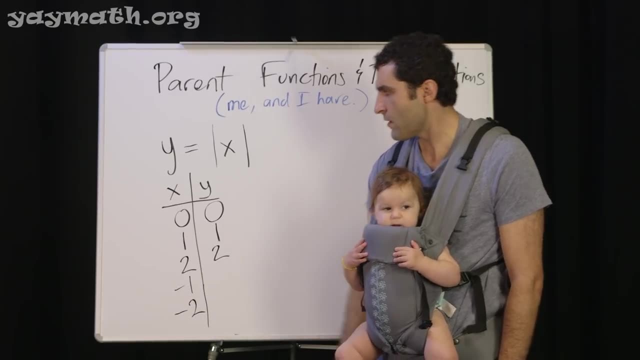 can try one. Absolute value of one for x is one. You could try two, and absolute value of two is two. negatives like negative one and negative two. There you go. What is the absolute value of negative one? if we were to put negative one in here, It would be one And the absolute. 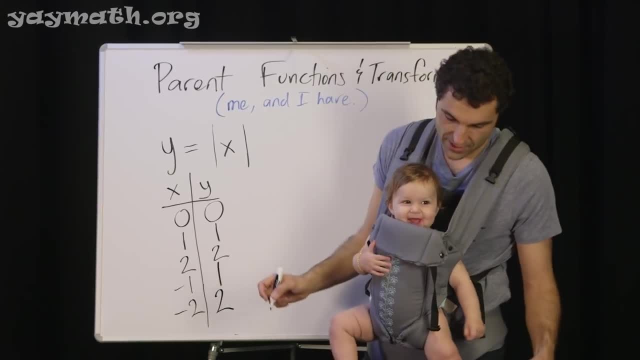 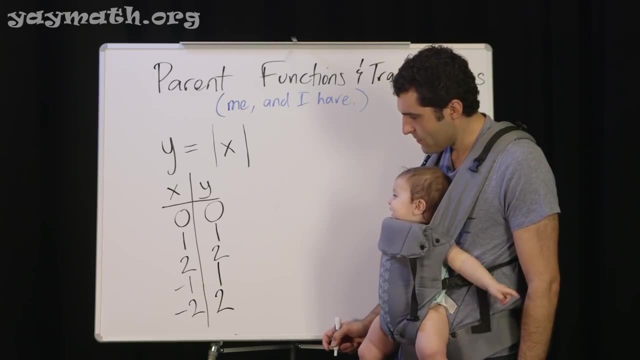 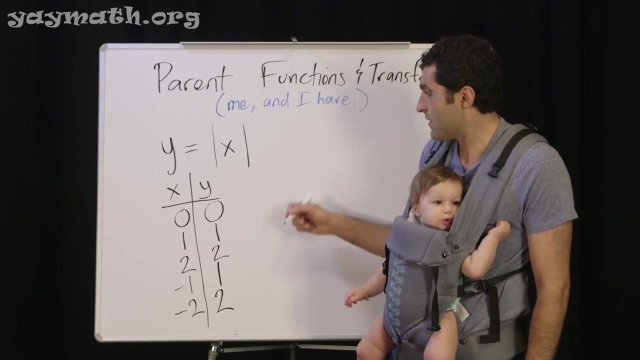 value of negative two would be two. That's right. Yeah, you want to keep going? Are you understanding it so far? I find it just as appealing as you do. I really do. But you know what It's going to get- even more insane. Let's do this. Yeah, take a good stretch, because 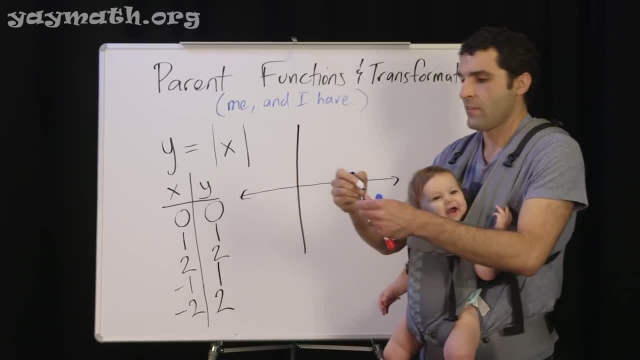 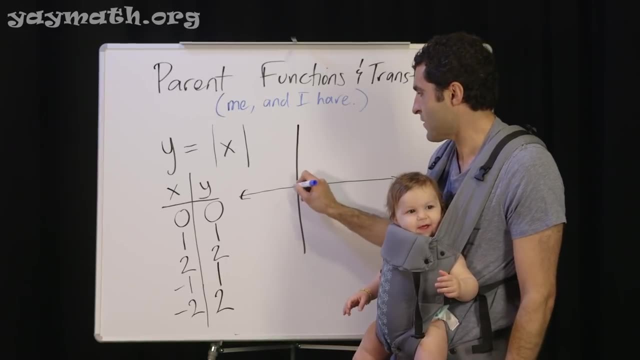 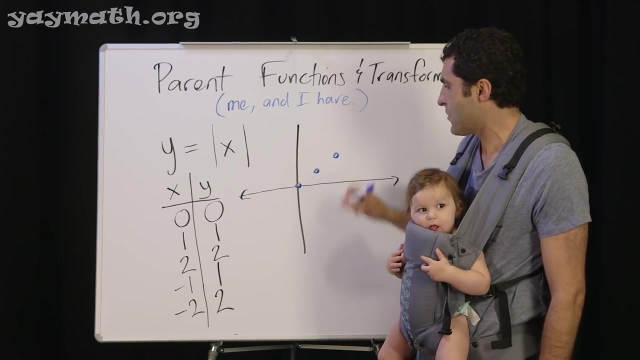 you're going to need it. Here it comes. Let's plot those points. Oh, thank you. This feels so nice. Your skin is insanely soft. I don't know how you do it. Do you use product or something I'm going to put in zero, zero, one, one, two, two, And then you have negative 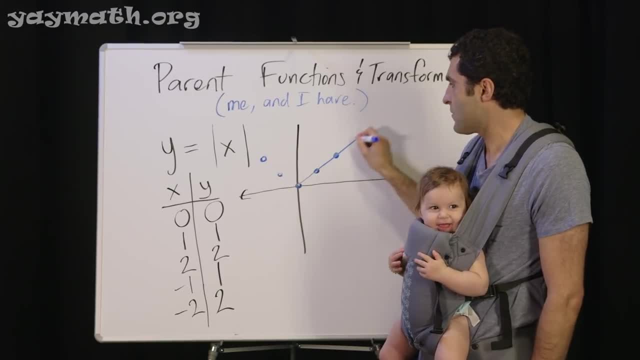 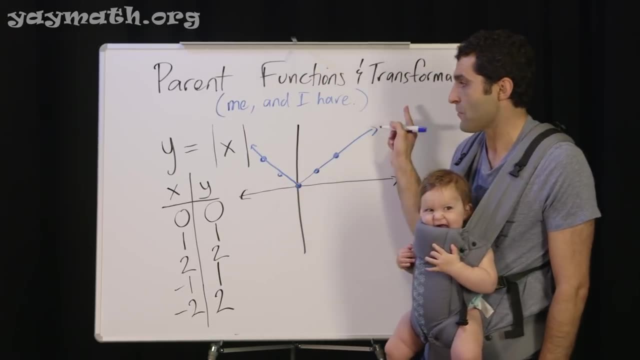 one, one and negative two, two. Absolute value looks like a V And the way I remember it with a V is negative one, one, two, two. And then you have negative one, one and negative two. What I love about this with my students is absolute value. There's your V for absolute. 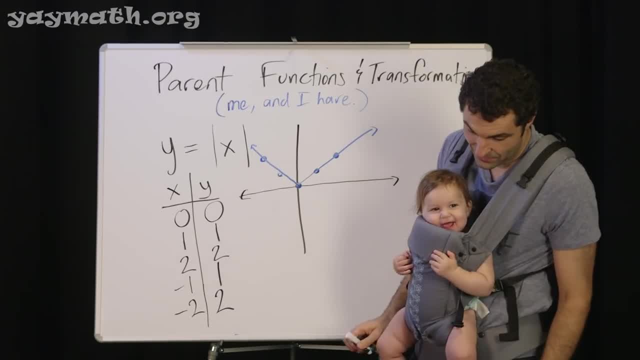 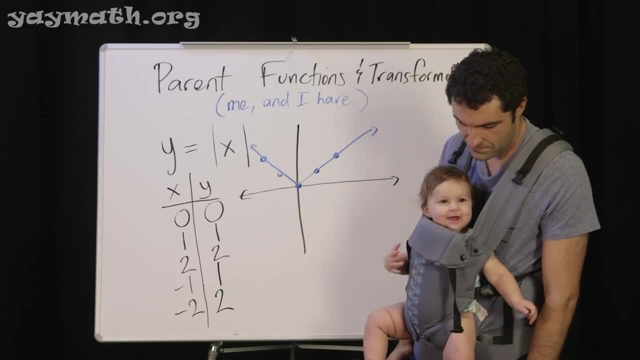 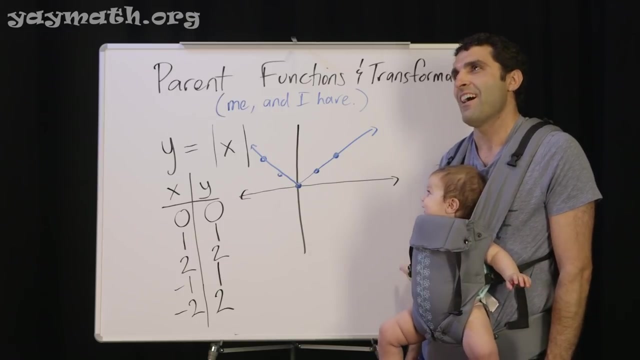 value. Now I know The thing about absolute value. what I really love is that everything stays positive. See how Y always results in a positive number. That's kind of like your mood right now. Oh, I love that sound. I really do. I really do. You are keeping it positive. 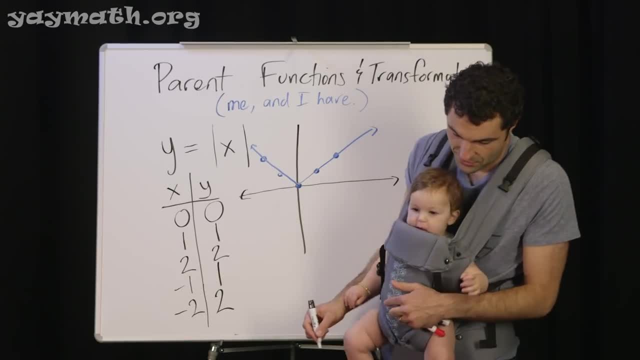 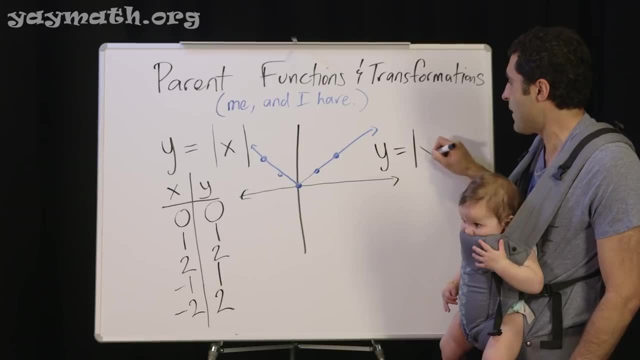 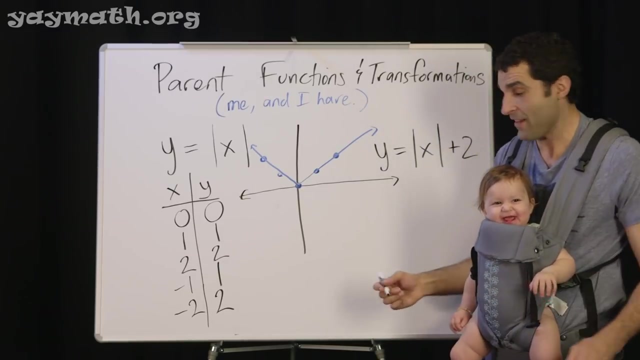 You are keeping it positive. That's a good character trait. I'm going to say that's biological. okay, so let's do some transformations on this action. what about absolute value of X plus 2? what would happen in this case? what would happen? let's find out, I know. 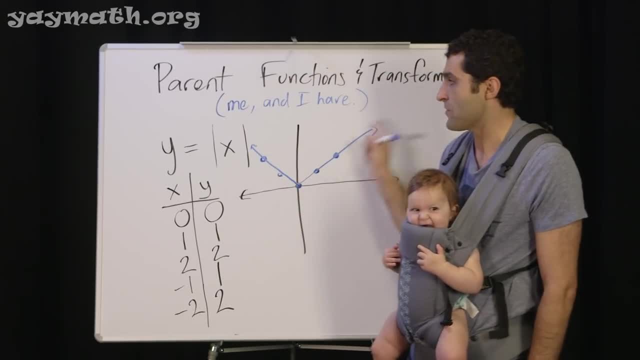 1, 1, 1, 1, 2, 2, and then you have negative 0, 0, 0, 0, 1, 0.. Absolute value. There's your V for absolute value. Now I know the thing about absolute. 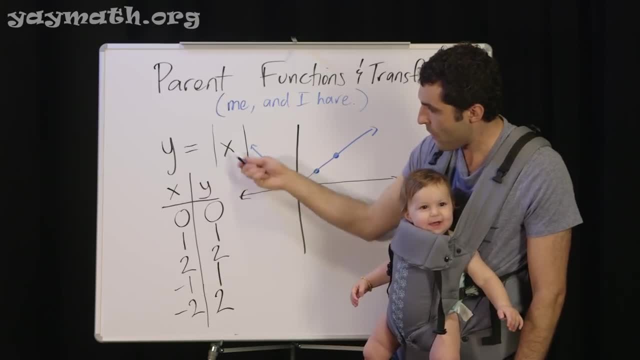 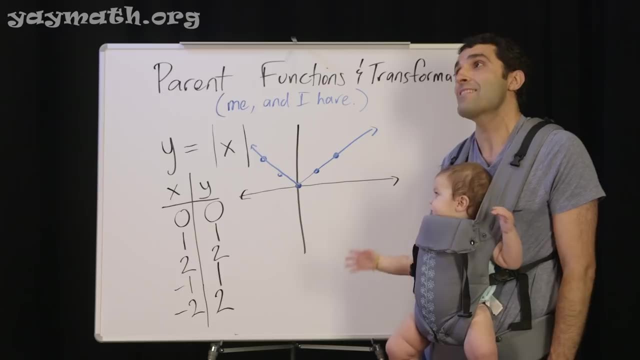 value. what I really love is that everything stays positive. See how Y always results in a positive number. That's kind of like your mood right now. Oh, I love that sound. I really do. I really do. You are keeping it positive. You are keeping it positive. 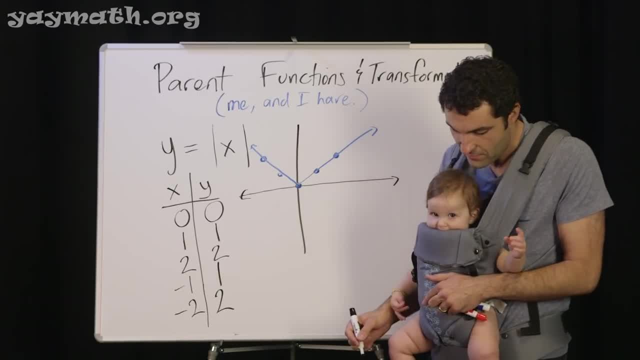 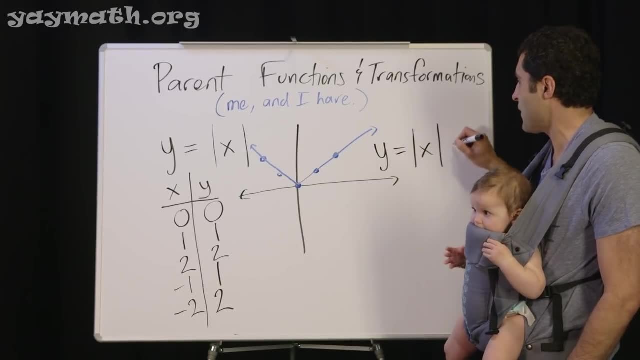 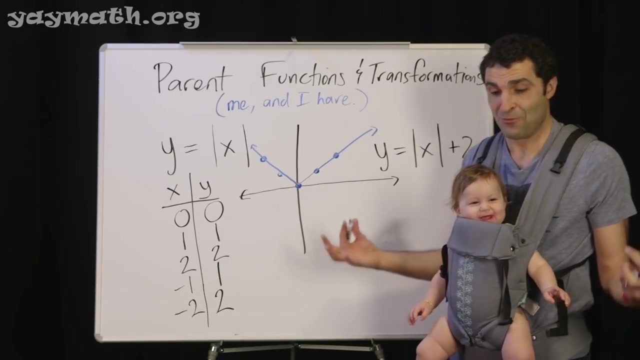 That's a good character trait. I'm going to say that's biological equal. okay, so let's do some transformations on this action. what about absolute value of X plus 2? what would happen in this case? what would happen? let's find out. I know I'm riveted with anticipation. let's do it. what if we? 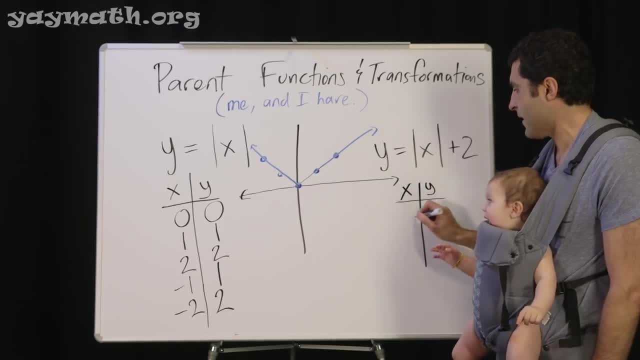 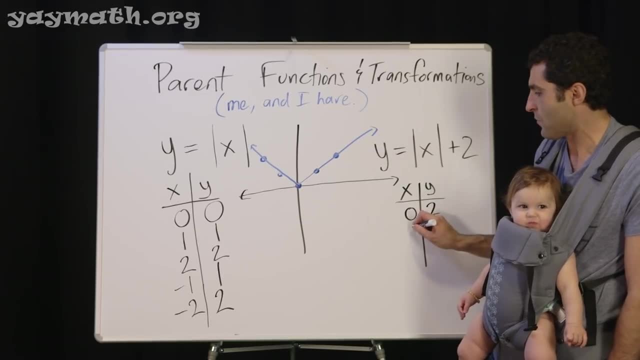 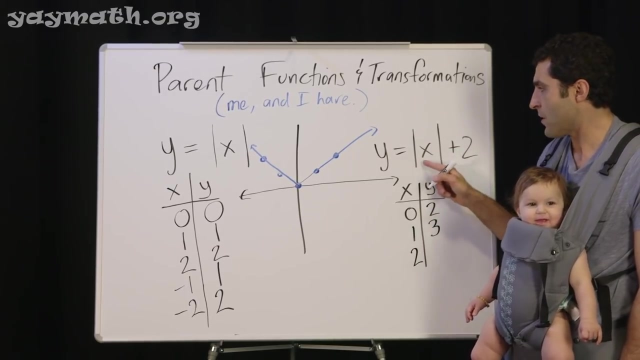 were to graph this. is it safe to say that if we plug in 0 for X, all right, and then add to it 2 to it, it becomes that if you plug in 1, 1, absolute value of 1 is 1 plus 2 is 3 and even 2. if we plug in 2 in here, we'll get 4. here's the. 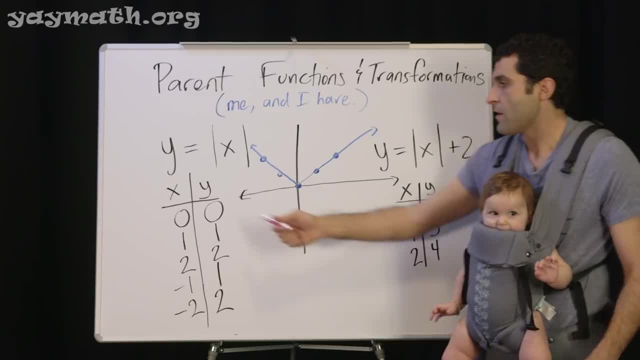 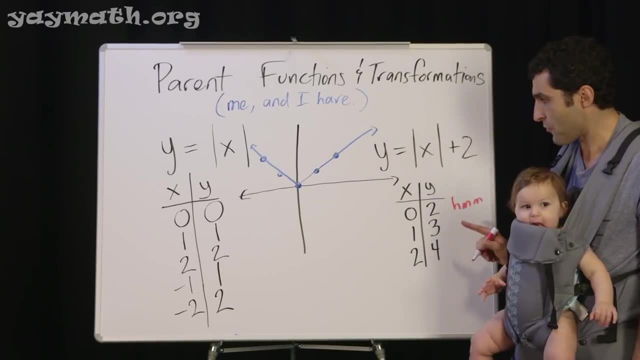 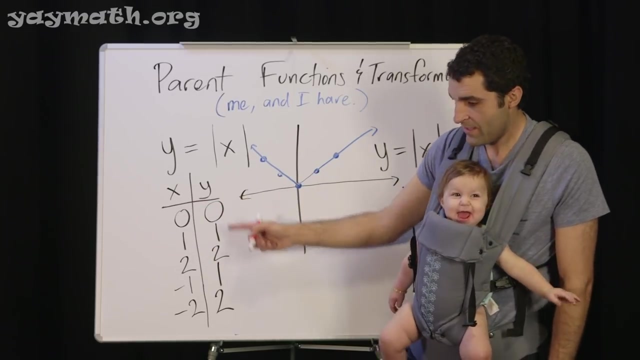 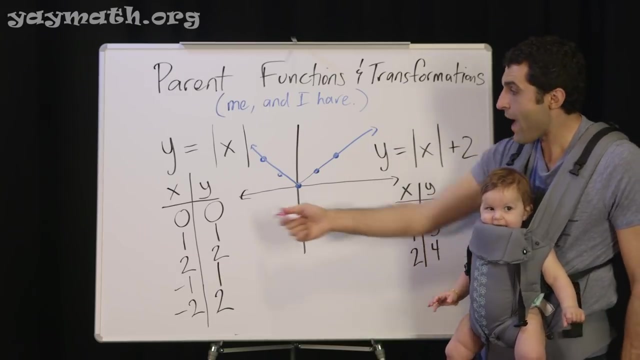 thing to keep in mind comparing these two: 0, 0, 0, 2. hmm, 1, 1, 1, 3. do you notice the difference? what happened here? do you see that X is the same, but now Y? it really did. it jumped that high. Y changed by 2 when you put 2 out here. so 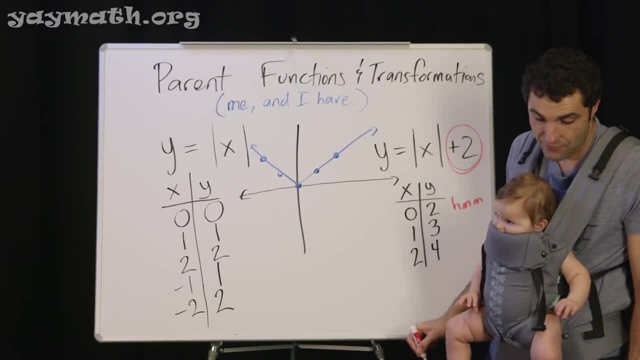 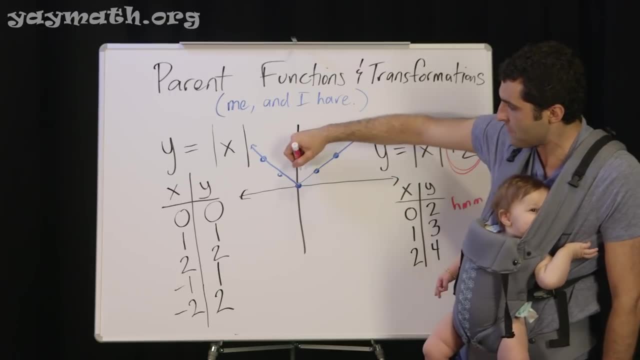 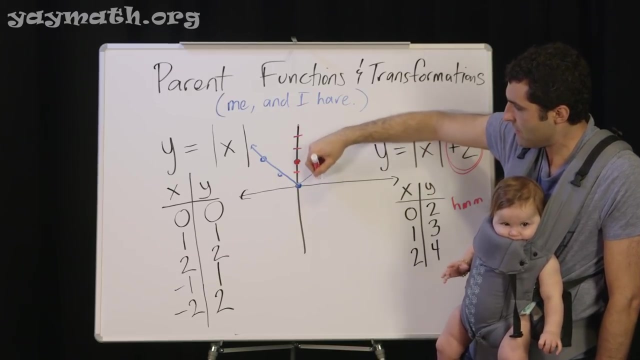 anytime you have a number out here, it moves the graph on Y. does that make sense? so let's actually graph that it's the same points. instead of 0, 0, we're doing 0, 2. so I go up 2. instead of 1, 1, we're going 1, 3. here it is. 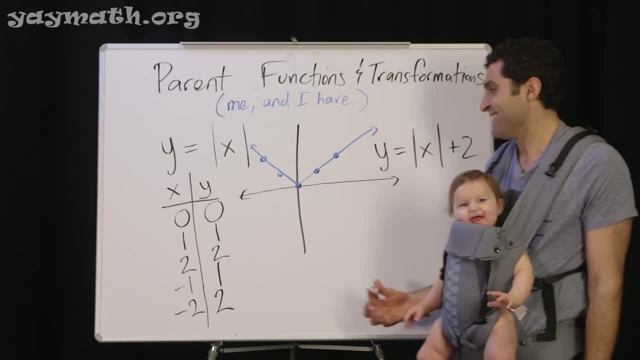 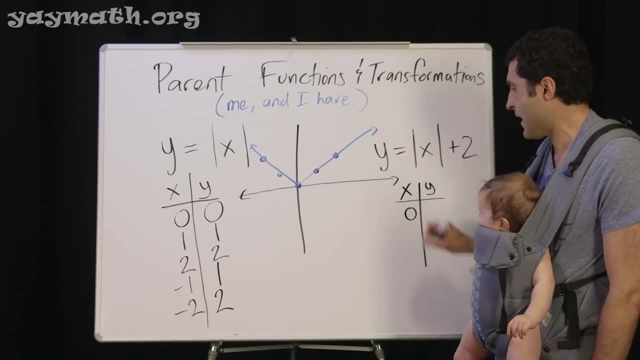 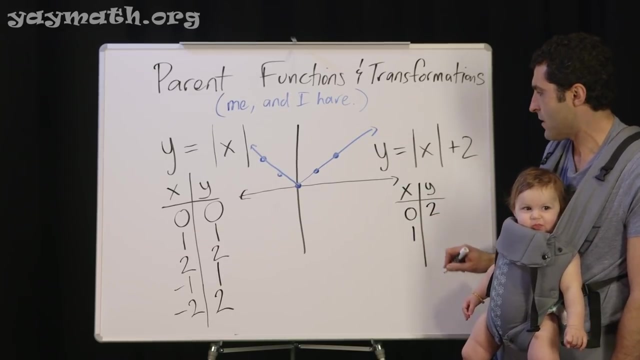 I'm riveted with anticipation. let's do it. what if we were to graph this? is it safe to say that if we plug in 0 for X, all right, and then add to it 2 to it, it becomes that if you plug in 1, 1, absolute value of 1 is 1 plus 2 is 3 and even 2? 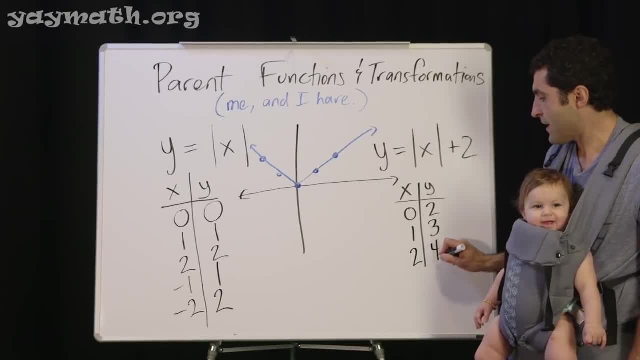 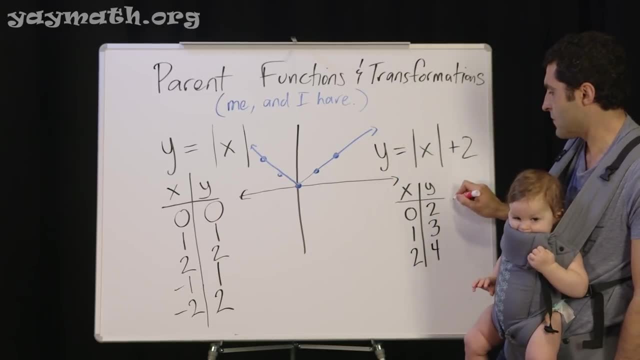 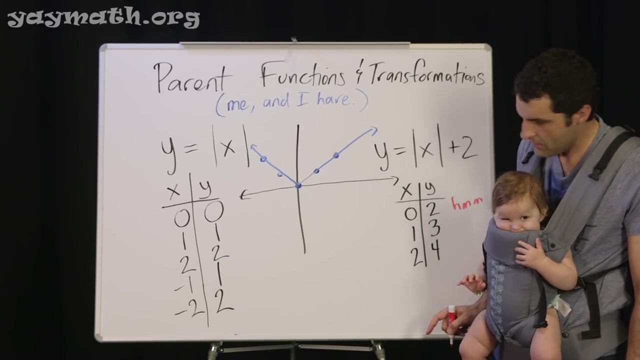 if we plug in 2 in here, we'll get 4. here's the thing to keep in mind comparing these two: 0 0, 0, 2. hmm, 1 1, 1, 3. do you notice the difference? what happened here? do you see that X is the same, but now Y? 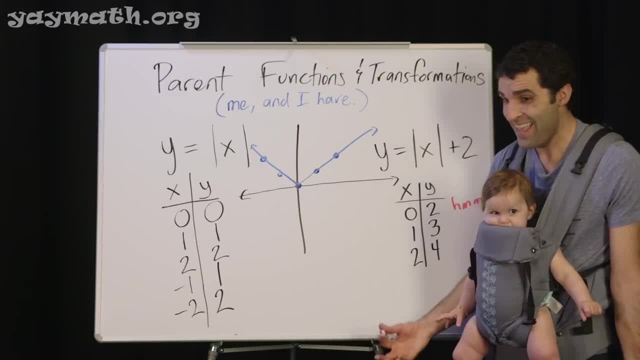 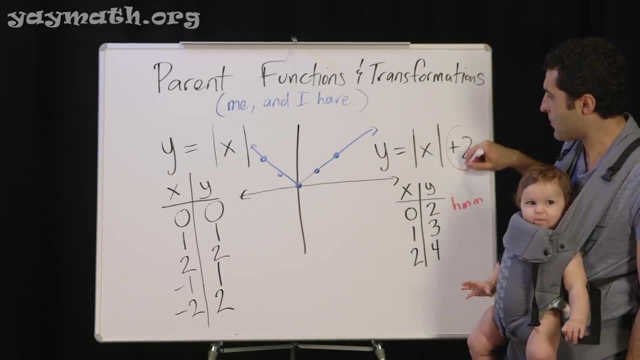 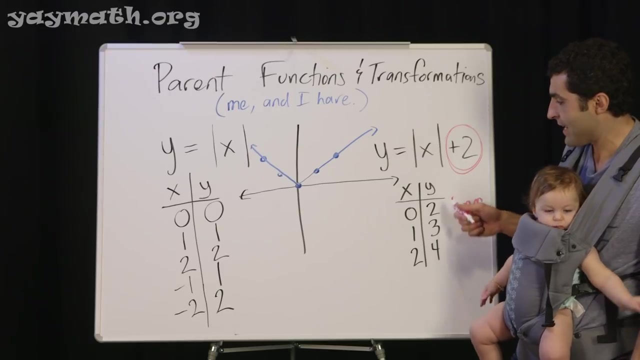 it really did. it jumped that high. Y changed by 2 when you put 2 out here. so anytime you have a number out here, it moves the graph on Y. does that make sense? so let's actually graph that it's the same points instead of 0, 0, we're. 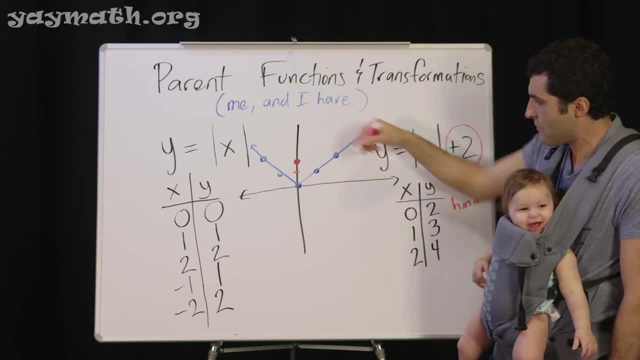 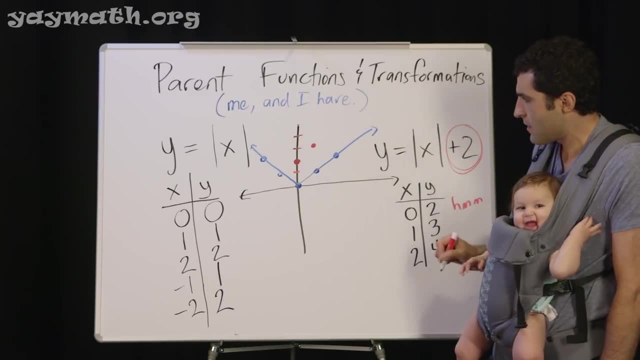 doing 0, 2, so I go up 2 instead of 1, 1. we're going 1, 3, here it is 1, 3. see that: 0, 2, 3, here it is 1, 3, here it is 1, 4, 5, 6, 7, 8, 9 and you'll get your same V shape. 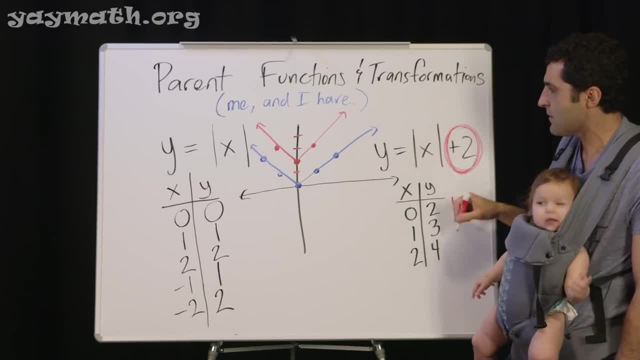 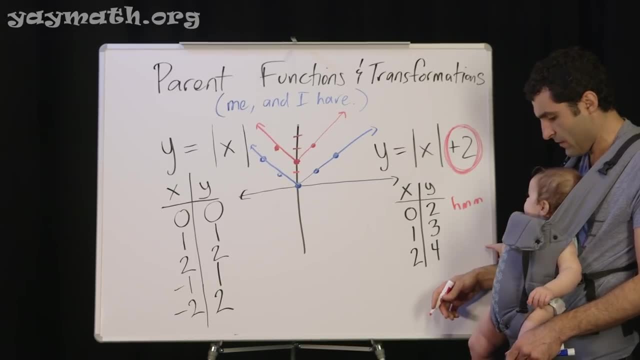 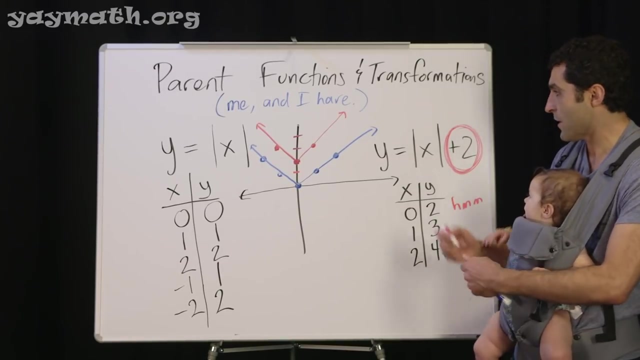 with the change vertically. so again, anytime you add or subtract out here, it goes up or down by that amount. yeah, check, check it out, make sure you get it. you don't want to actually throw the board down. okay, that's what happened last week. all right, I used to have you recovered from that emotionally. 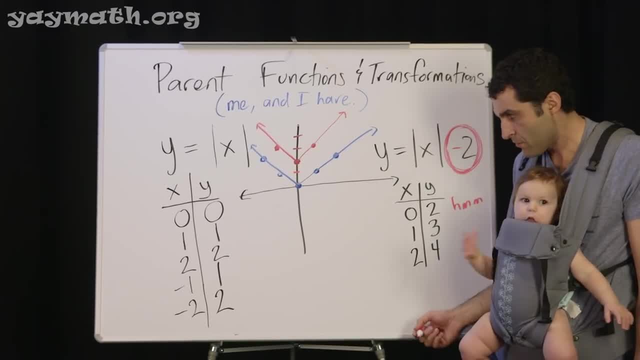 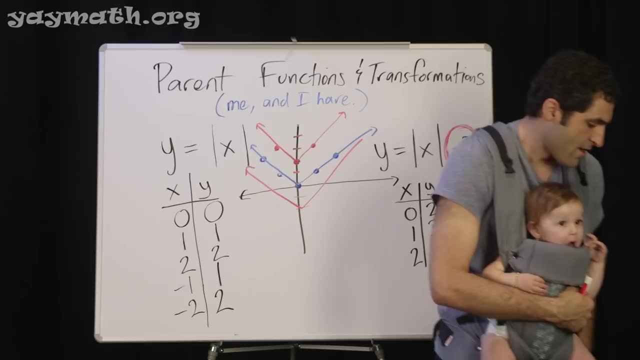 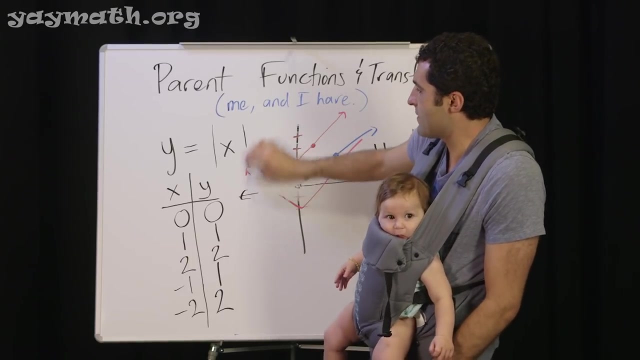 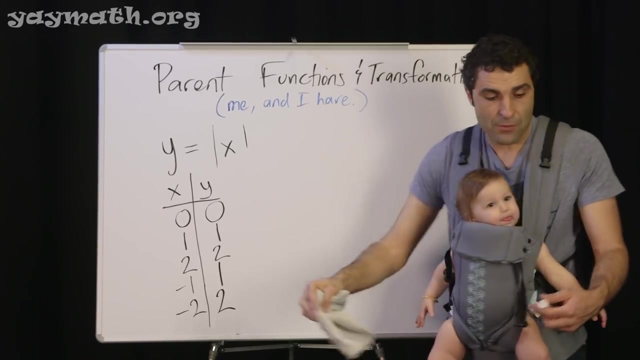 apparently you have, so let's do it. if it was like, let's say, minus 2, do you agree? would be like there, so far, so good. all right, a few more transformations. buddha, buddha. gotta check out the yoga legs. i know we'll take this off. we'll add a new graph. all right, now what we're. 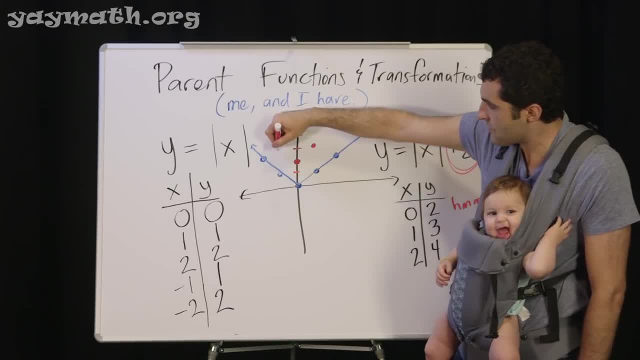 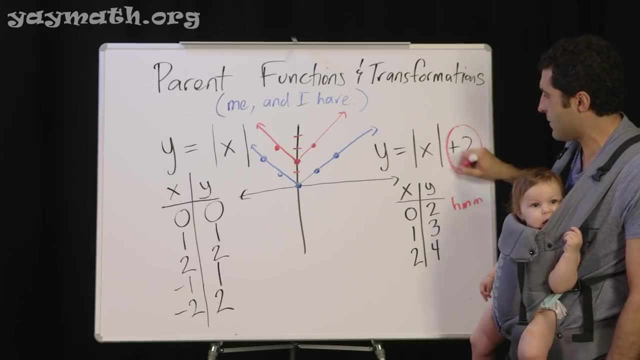 1, 3. see that and you'll get your same V shape with the change vertically. so again, anytime you add or subtract out here, it goes up or down by that amount. yeah, check, check it out, make sure you get it. you don't want to actually throw. 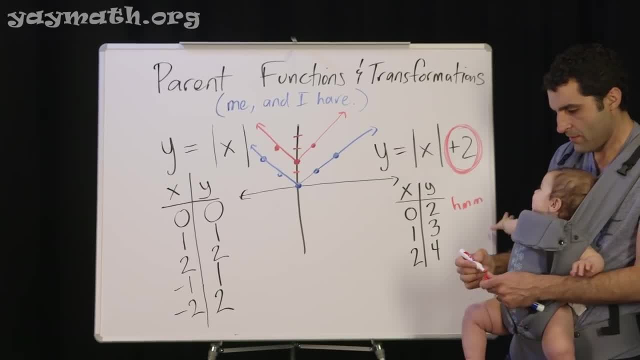 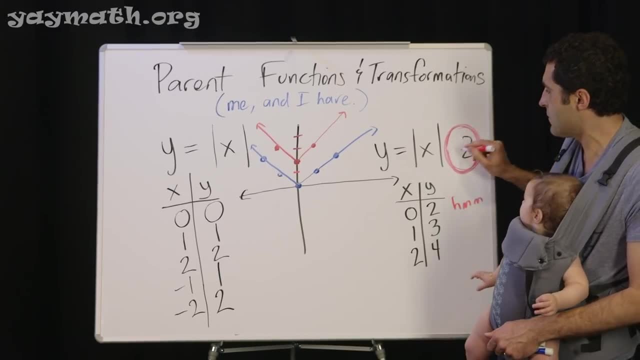 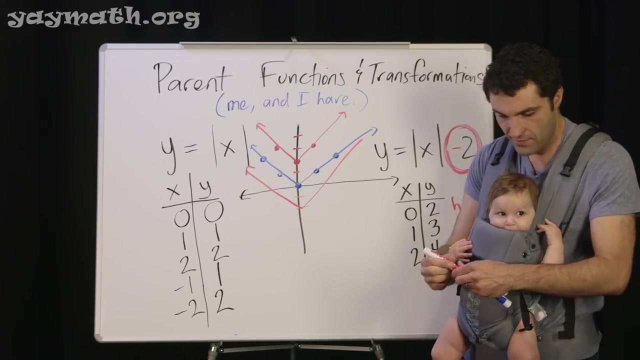 the board down. okay, that's what happened last week. all right, I used to have you recovered from that emotionally. apparently you have, so let's do it. if it was like, let's say, minus 2, do you agree? that would go down to 1. 2 would be like there. so far, so good. all right, a few more transformations. 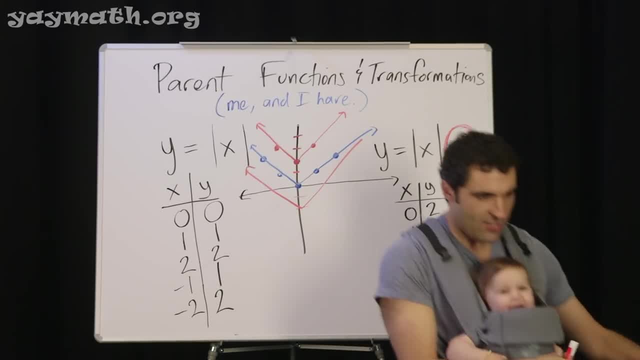 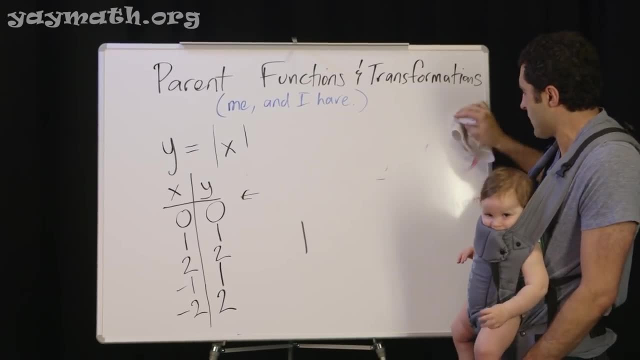 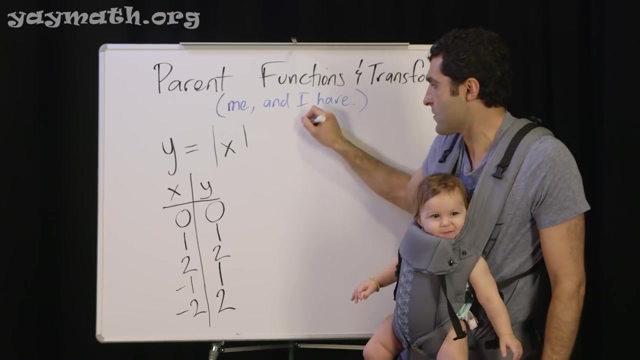 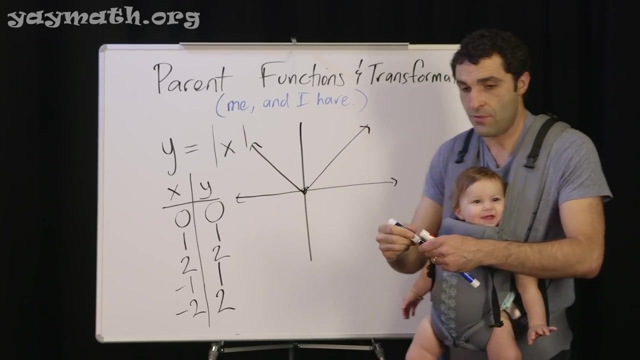 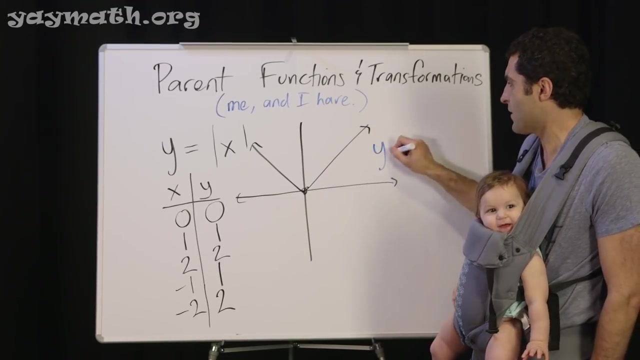 Buddha, Buddha, gotta check out the yoga legs. I know we'll take this off. we'll add a new graph. all right, now, what we're gonna do is what if we did? here's your original parent function absolute value graph there in black, and let's do a new one in blue. you're so happy right here? y equals, let's say X. 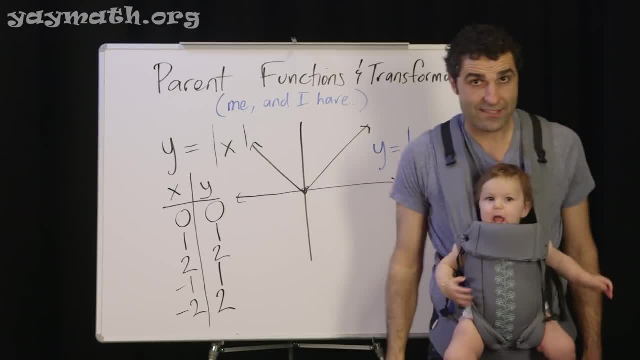 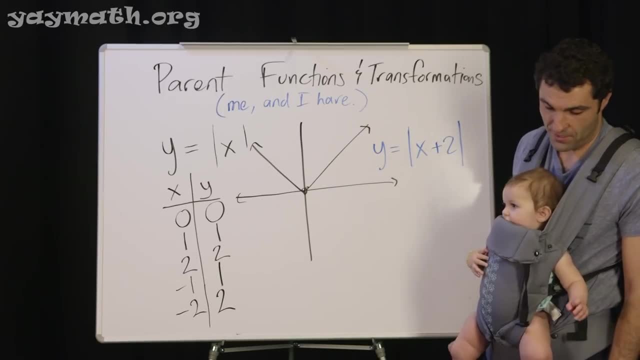 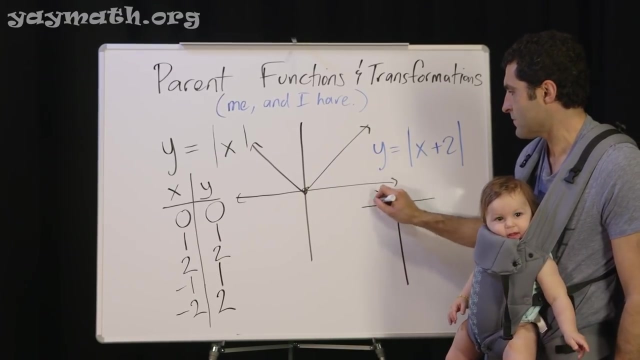 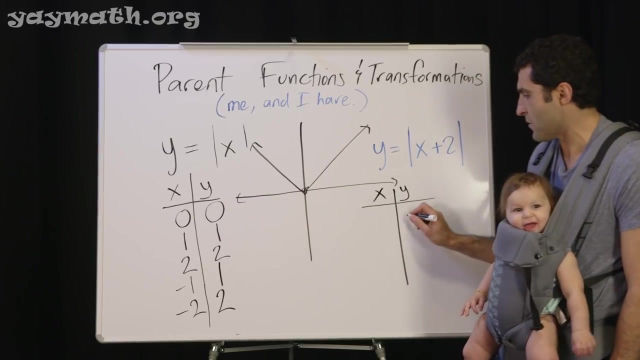 plus 2 inside. what would that do? what would that do? your sounds soothe me. I love them so much. now let's put in our table. see what happens. okay, now I want you to think. think this through: if I wanted Y to be 0, just bear. 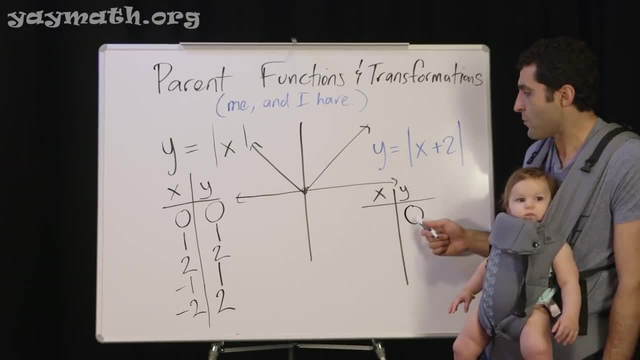 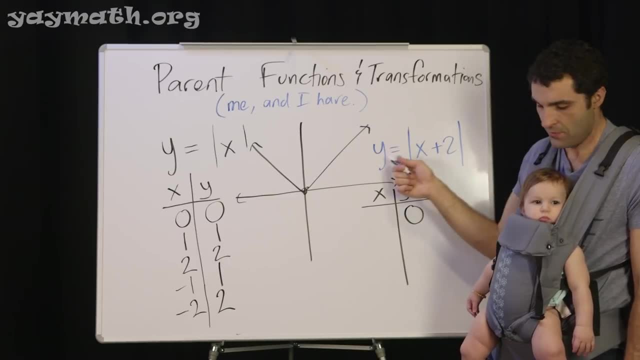 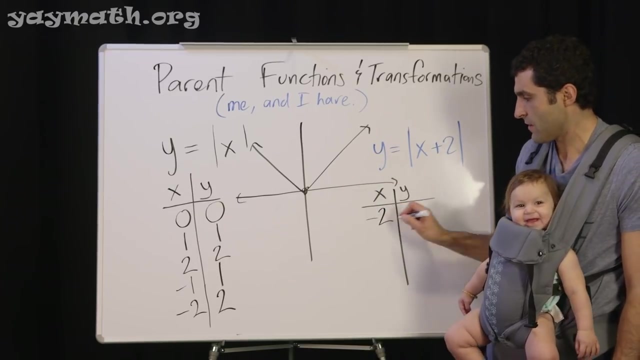 with me for a second. okay, you're patient, right? if I wanted Y to be 0 again, what would X have to be? what could I plug in here so that when I add 2, it results in 0? yes, that's right. yes, we are connected. you approve, it is negative 2. it is negative 2. 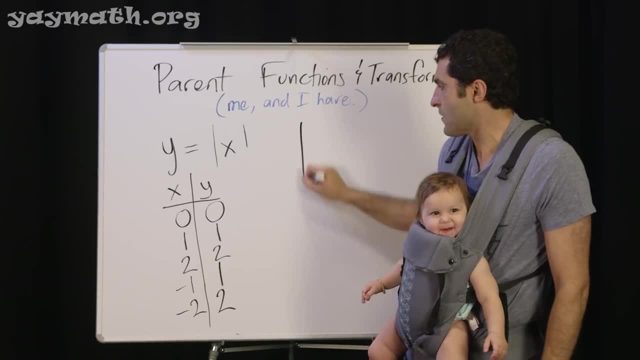 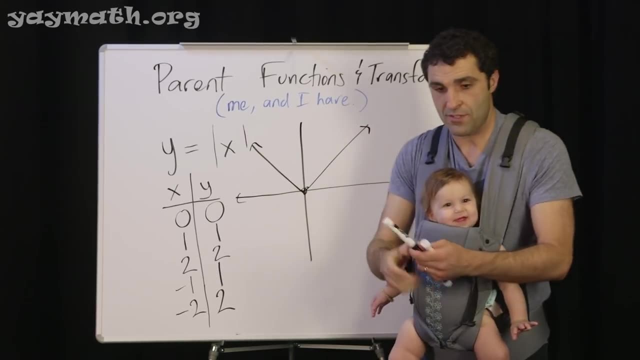 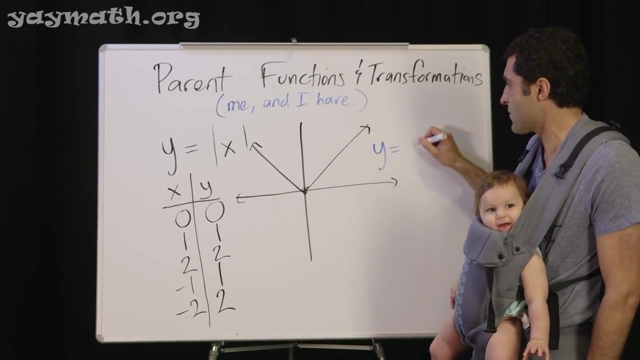 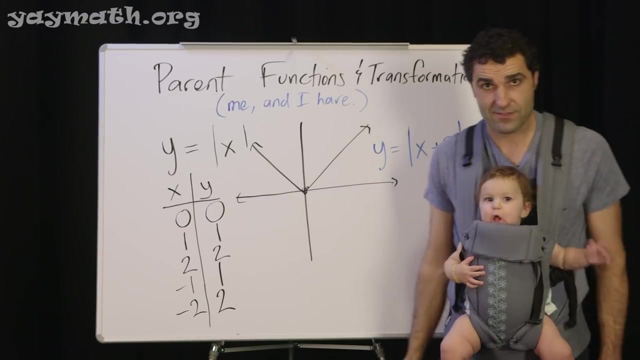 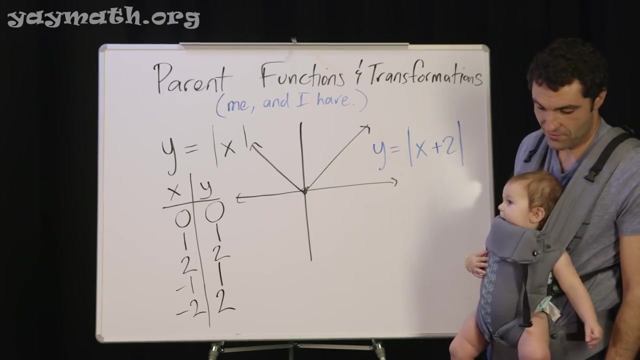 gonna do is what if we did? here's your original parent function absolute value graph, there in black. let's do a new one in blue. you're so happy right here. y equals, let's say, x plus 2 inside. what would that do? what would that do? your sounds soothe me. I love them so much. now let's put in. 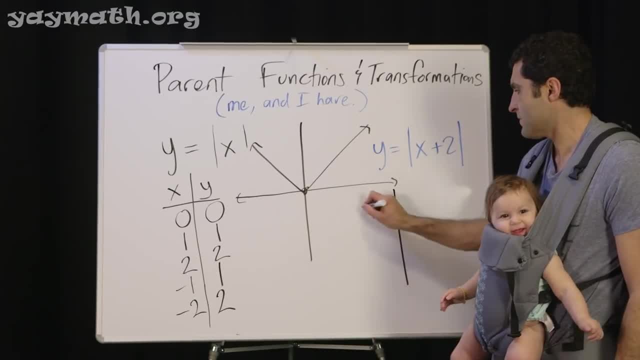 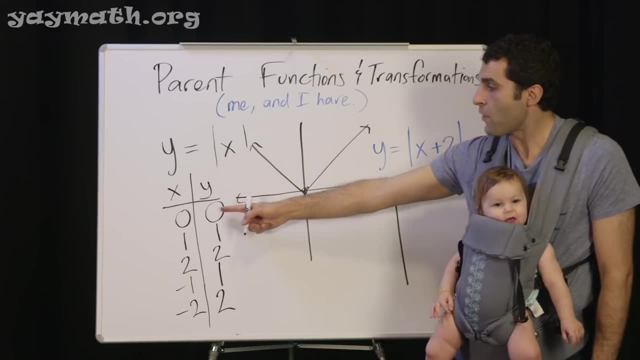 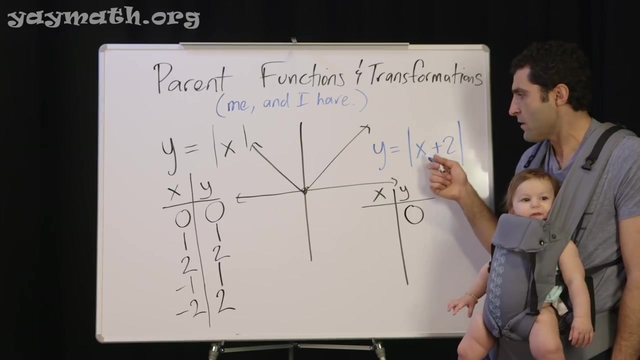 our table. see what happens. okay, now I want you to think. think this through. if I wanted y to be 0, just bear with me for a second. okay, you're patient, right? if I wanted y to be 0 again, what would X have to be? what could I? 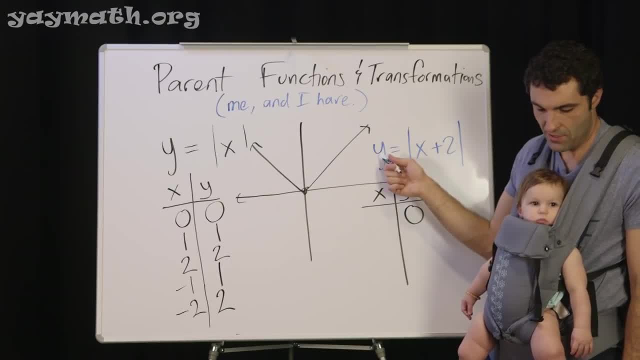 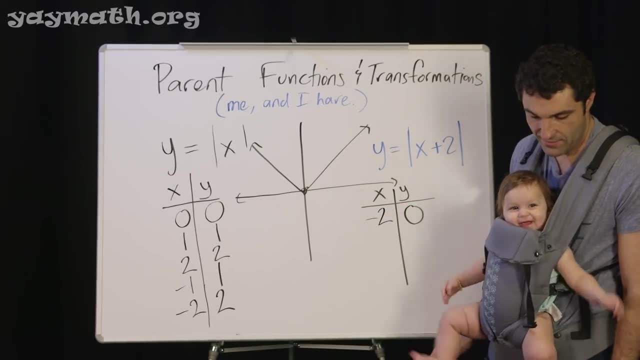 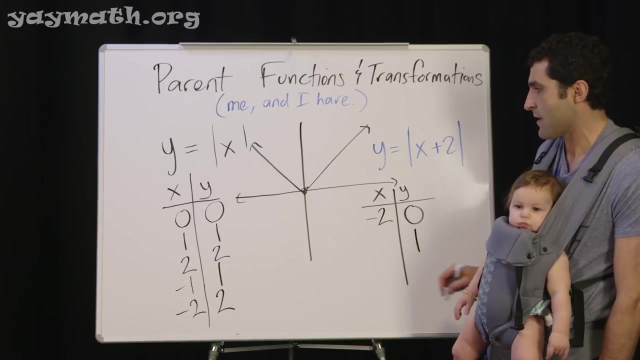 plug in here so that when I add 2 it results in 0. yes, that's right. yes, we are connected. you approve it. it is negative 2. it is negative 2, right. and what if I said 1 over here, matching up this point to this point, if I wanted. 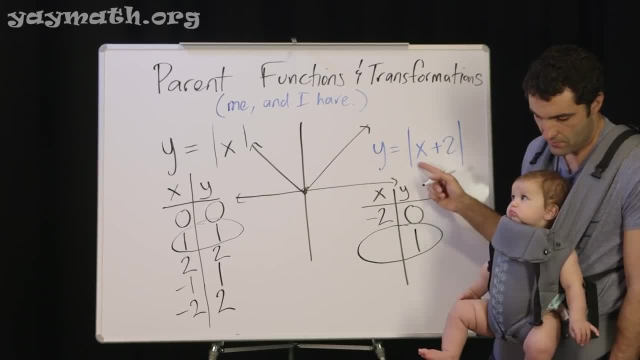 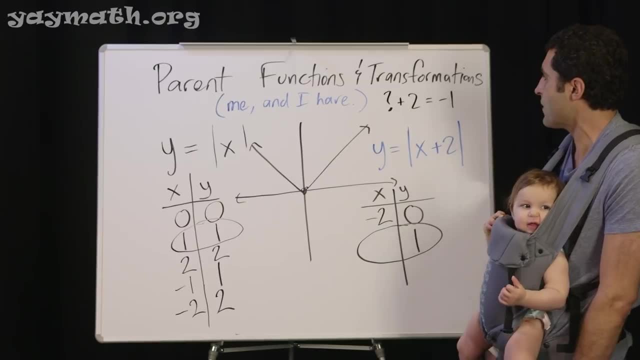 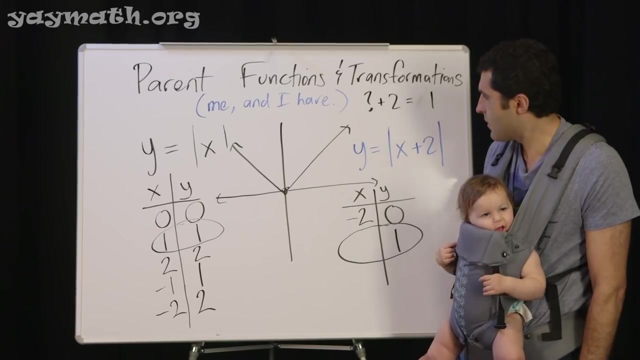 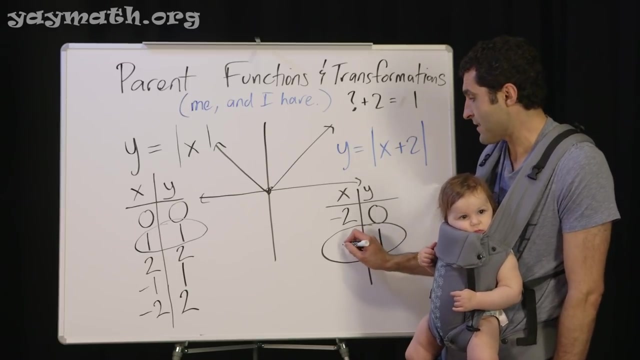 y to result in 1. what would X have to be? now? what plus 2 will even write it. what plus 2 equals negative 1 or, excuse me, 1. you think that through what plus 2 equals 1? okay, yeah, I guess I stumped you on that one. that's going to be negative 1. the point is what ends up. 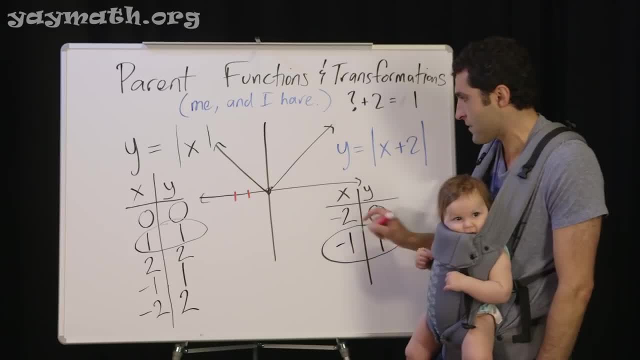 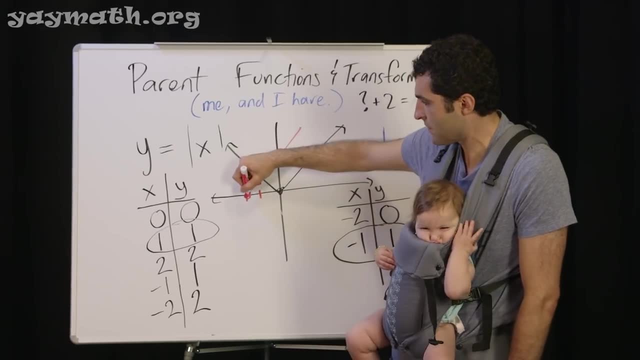 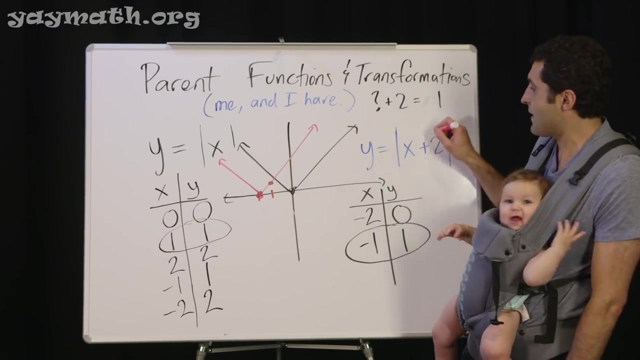 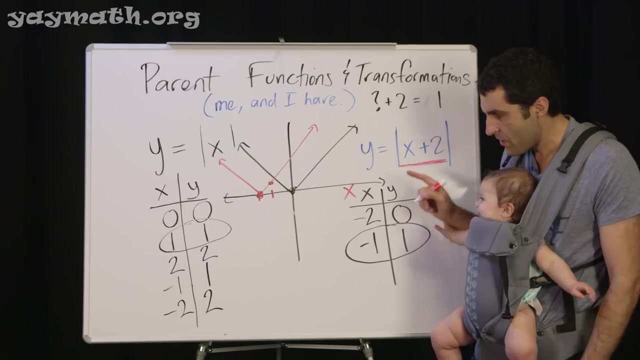 happening is that it moves left. see that negative 2, 0, negative 1, 1. and we got this effect here, which is really strange to me, as a form of transformation, because you'd think that plus 2 would move it right to. it's an X transformation. do you see how it's inside here partying with the X? you see that? 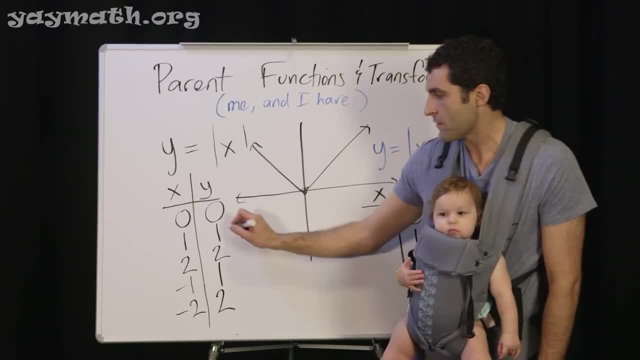 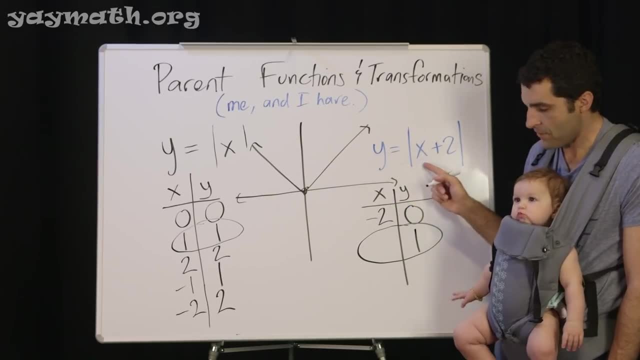 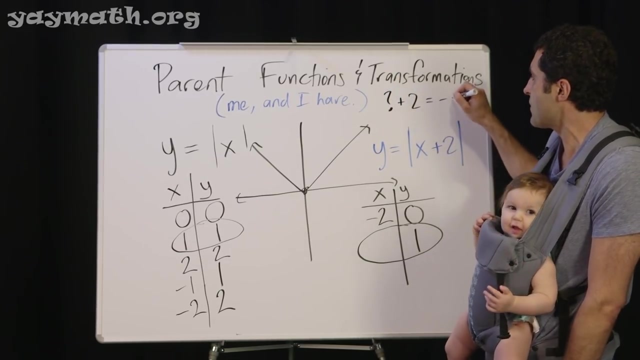 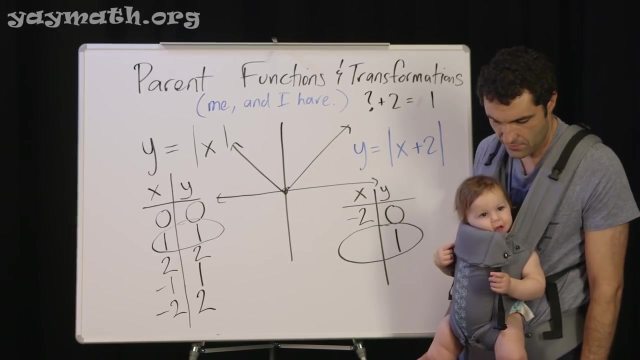 right. and what if I said 1 over here, matching up this point to this point? if I wanted Y to result in 1, what would X have to be now? what plus 2 will even write it. what plus 2 equals negative 1, excuse me, 1. you think that through what? 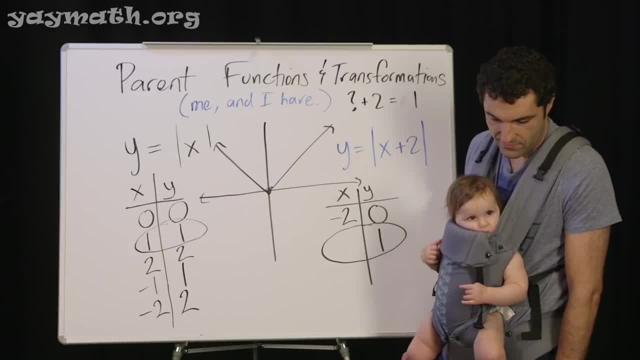 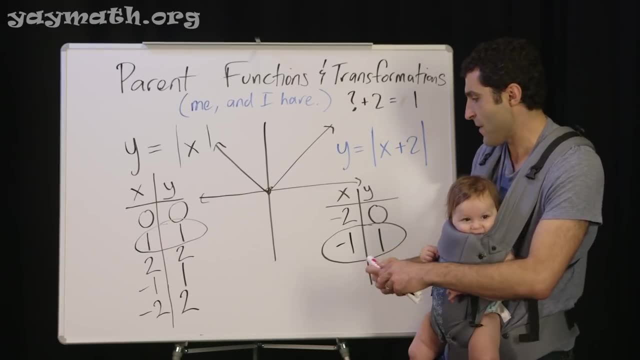 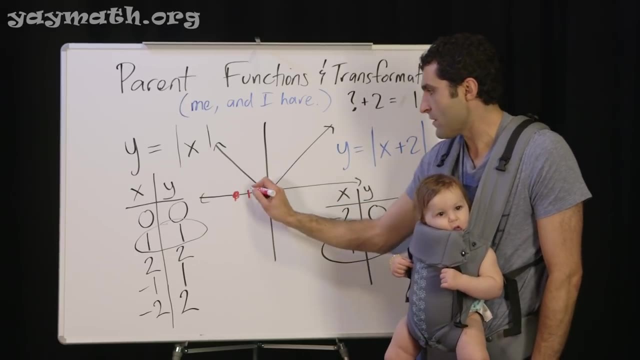 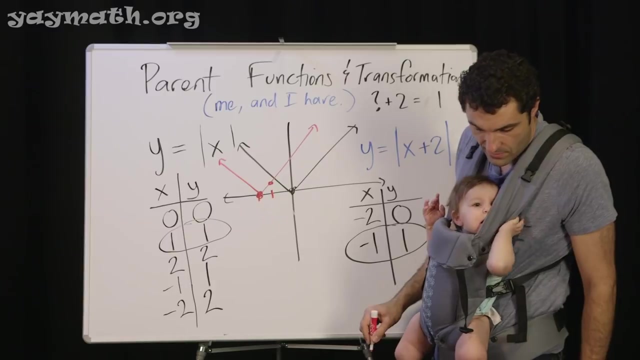 plus 2 equals 1. okay, yeah, I guess I stumped you on that one. that's gonna be negative 1. the point is, what ends up happening is that it moves left. see that negative 2, 0, negative 1, 1, and we got this effect here, which is really strange to me as a form. 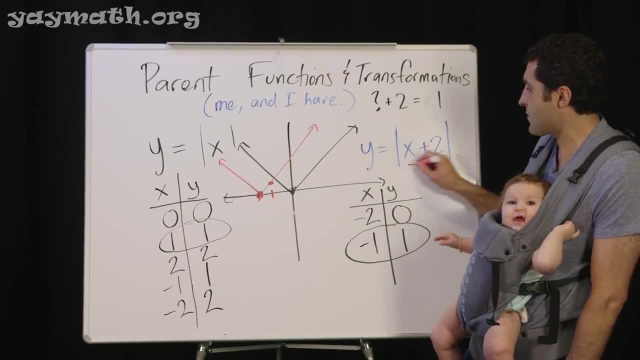 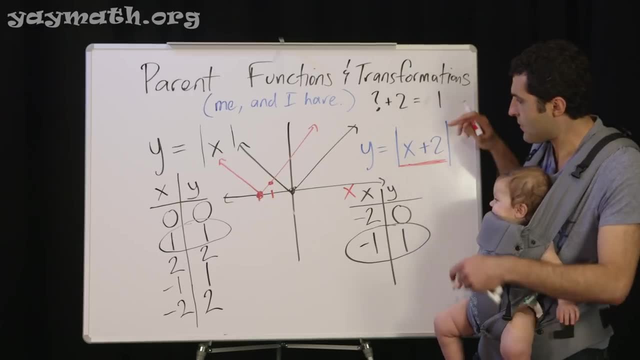 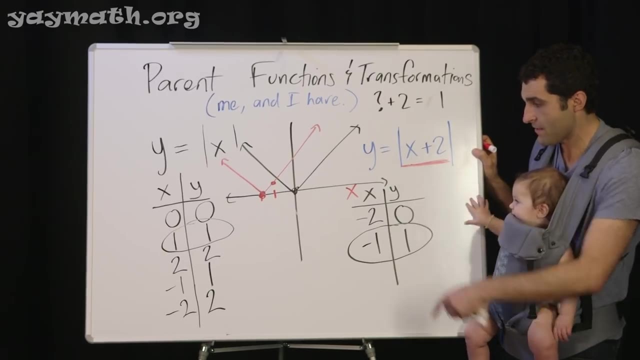 of transformation, because you'd think that plus 2 would move it right to, because in it's an X transformation. do you see how it's inside here partying with the X? you see that. see it's partying with the X there. so you think it affects X and that's. 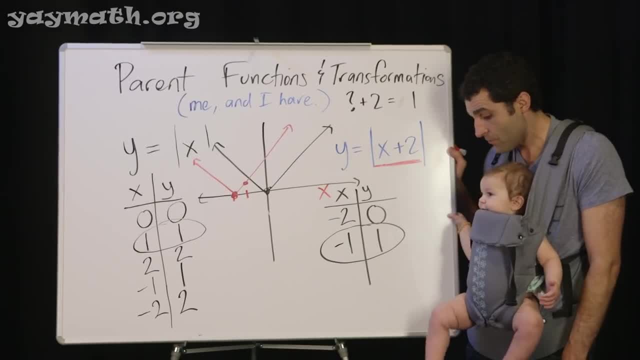 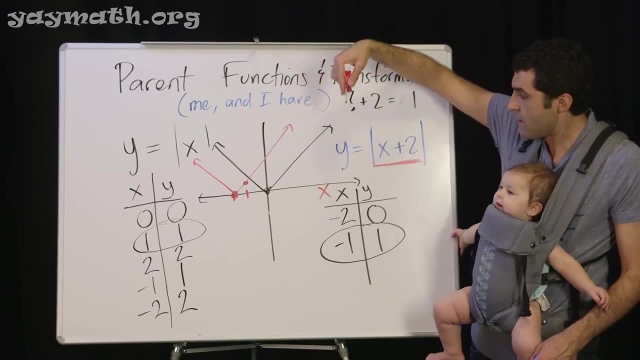 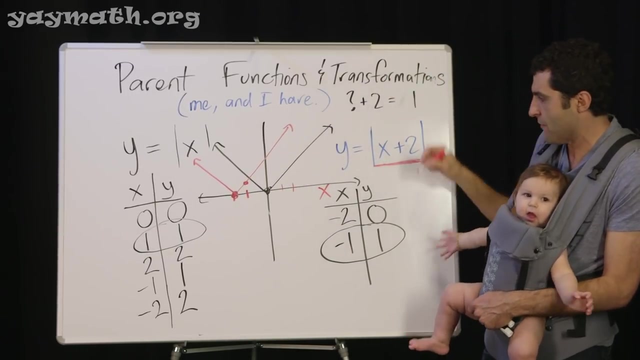 true, it does affect X, but what's really important to keep in mind is that it's not- and hold on, I'll give you a chance for questions. it's not really plus 2 this way. you'd think it would be right to, but it has this sort of opposite. 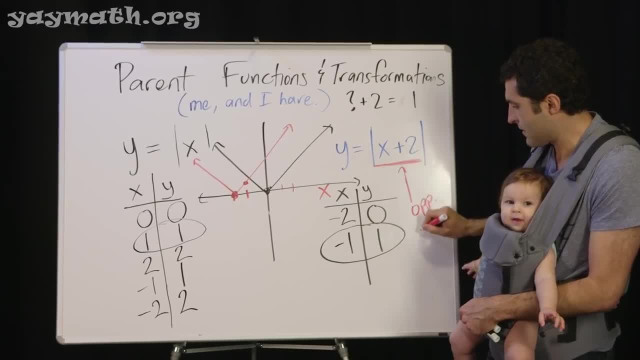 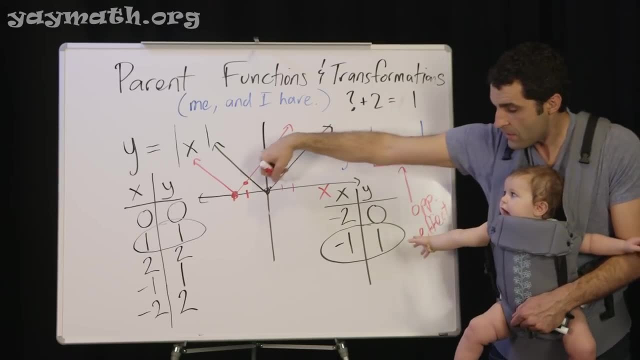 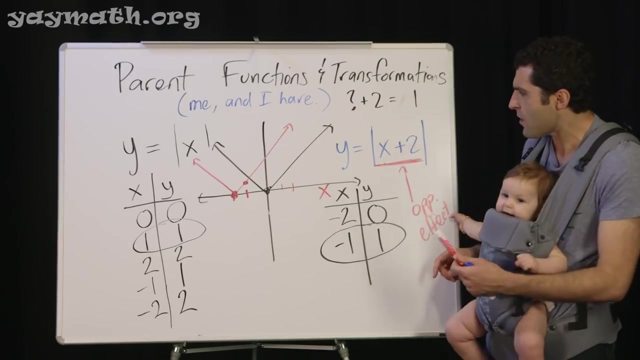 effect. here it has an opposite effect. so if you see that it goes plus 2 inside, it actually moves to the left on the graph. does that make sense? yeah, I know it is sort of disturbing. when I first learned this I was like, oh, it's in with X, it's plus 2. 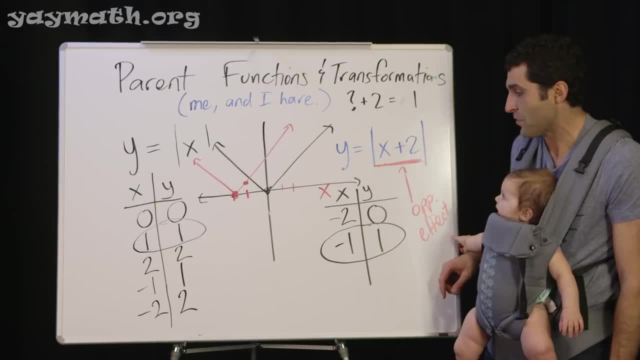 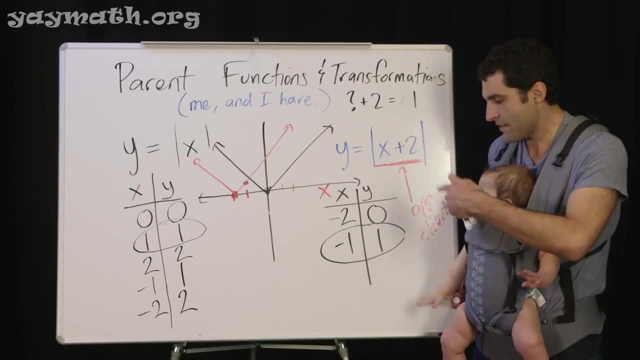 you should move it right to. but then the points don't actually line up when you plug it in, because you'll see that negative 2, 0 is the point to actually plug in. right, yeah, you can. you can erase that, because I'm sort of disgruntled by: 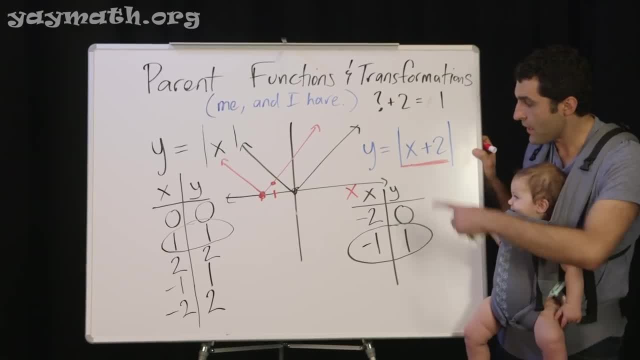 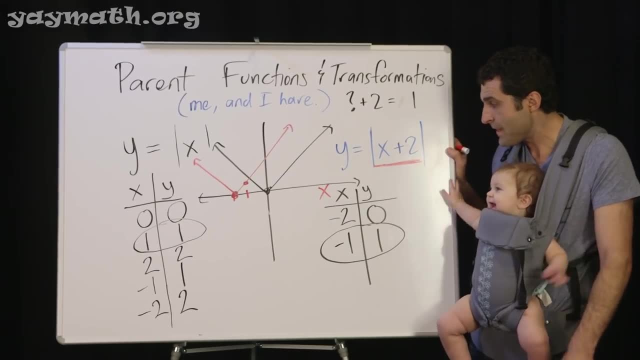 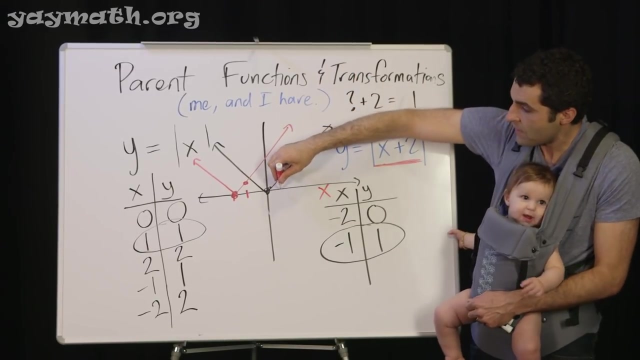 see it's partying with the X there. so you think it affects X, and that's true. it does affect X, but what's really important to keep in mind is that it's not- and hold on, I'll give you a chance for questions. it's not really plus 2 this way. you'd think it would be right 2, but it has this sort of 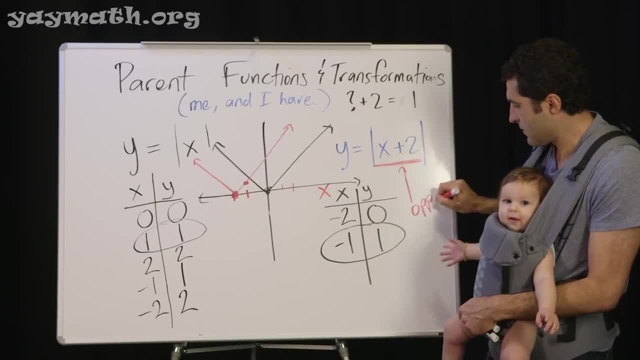 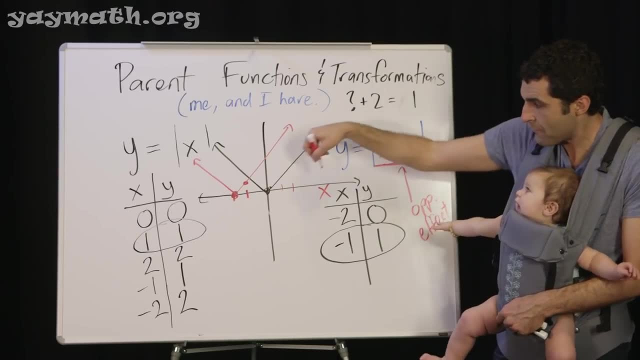 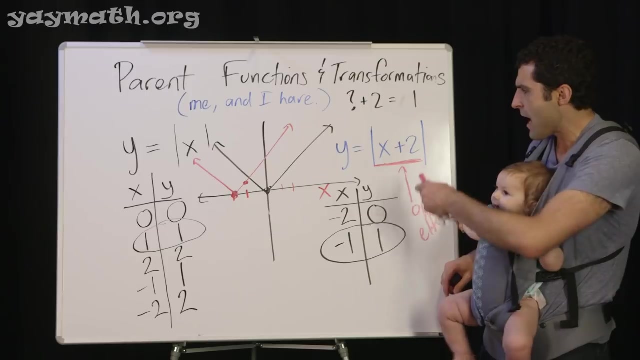 opposite effect. here it has an opposite effect. so if you see that it goes plus 2 inside, it actually moves to the left on the graph. does that make sense? yeah, I know it is sort of disturbing. when I first learned this I was like, oh, it's in with X, it's plus 2. you should move it right too. but then the points. 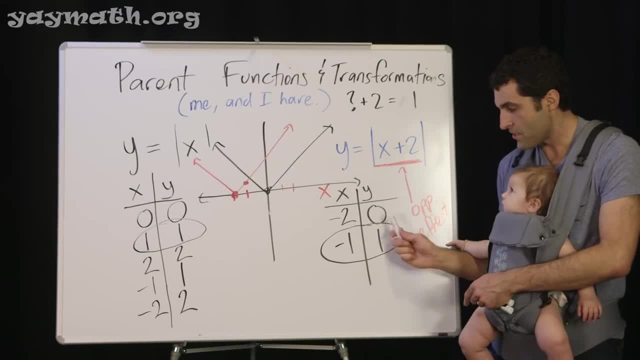 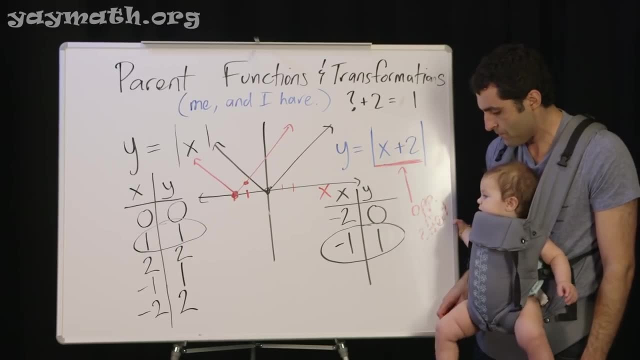 don't actually line up when you plug it in, because you'll see that negative 2, 0 is the point to actually plug in, right, yeah, you can. you can erase that, because I'm sort of disgruntled by it as well. yeah, it's weird that it goes opposite when it's inside with X, but can you recover from that? 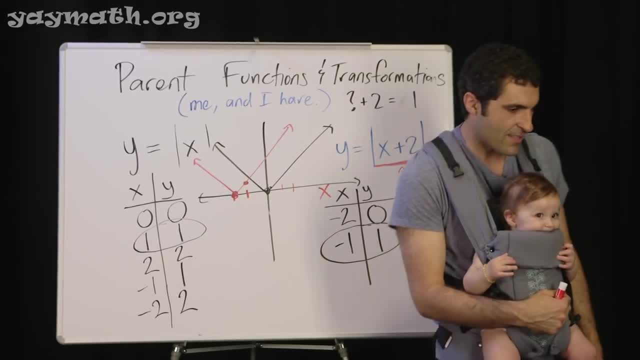 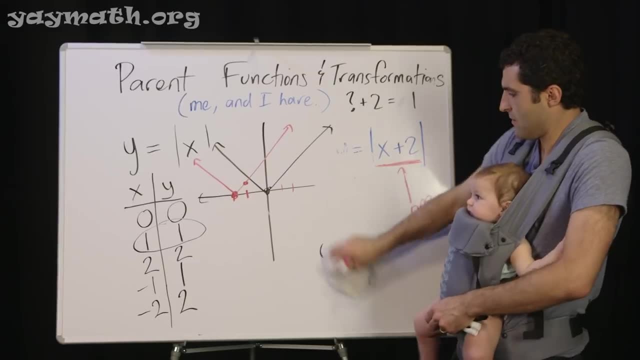 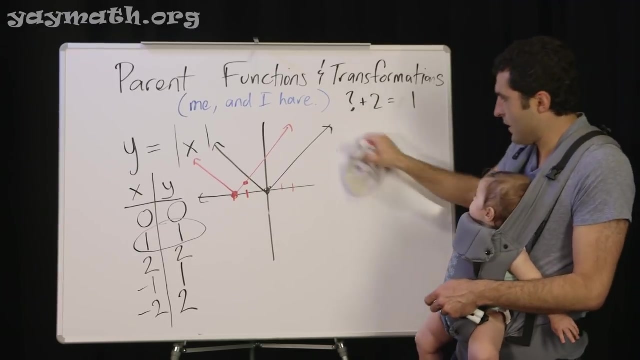 okay, I'm glad, I'm glad. a few more transformations. let me get down to Buddha Buddha, a baby Buddha, Buddha, baby, hit that off. I know, yeah, you feel the bicep. it's all because of you, all because of you. you gotta learn to walk one of these days. but you know I'm not rushing you. I'm not rushing you. 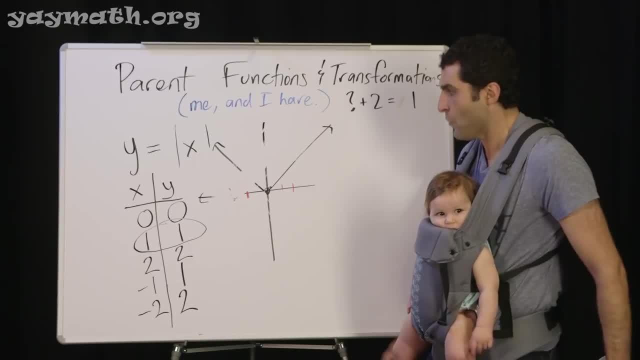 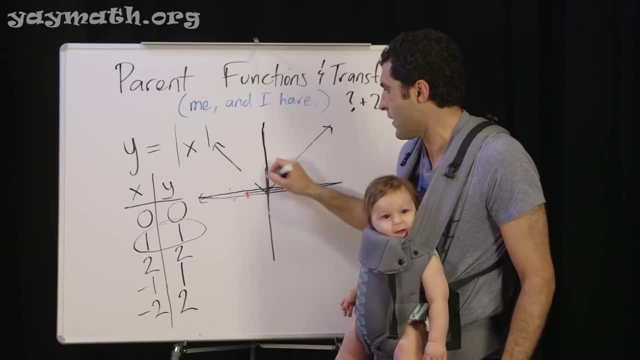 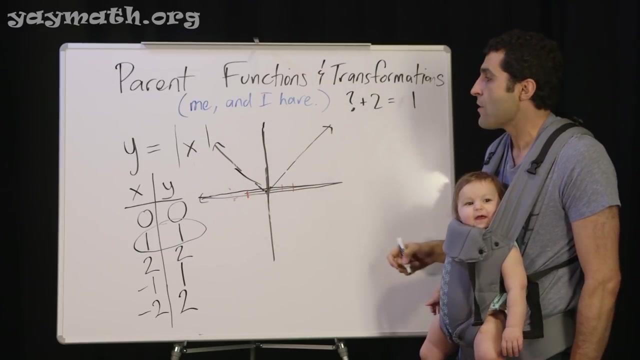 everyone's got to learn it their own pace right Now, focus. Okay, so there you go. The next transformation we did outside is up down. We did inside is left right but opposite right. The next one has to do with making it negative. 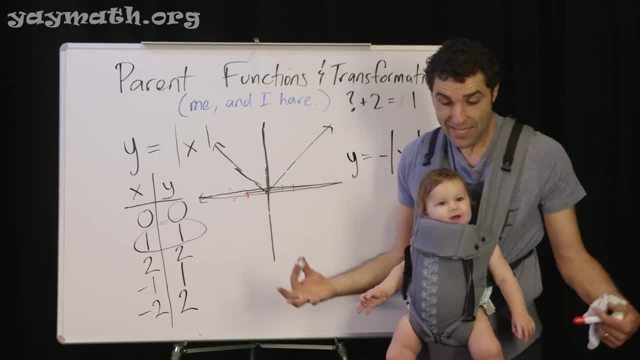 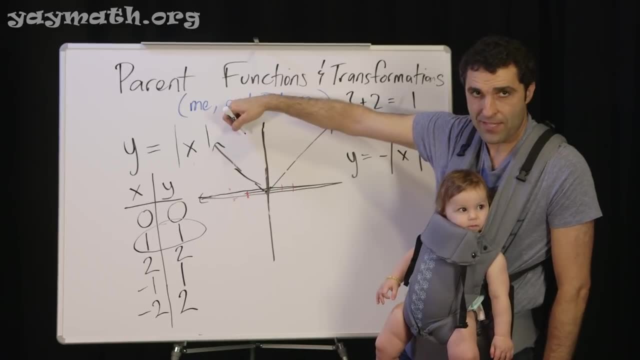 What's good about this is that these transformations apply to all parent functions, all parent functions. So if you go out here plus or minus something, it'll always go up down. If you go inside left or right something, it'll always go left or right, but opposite. 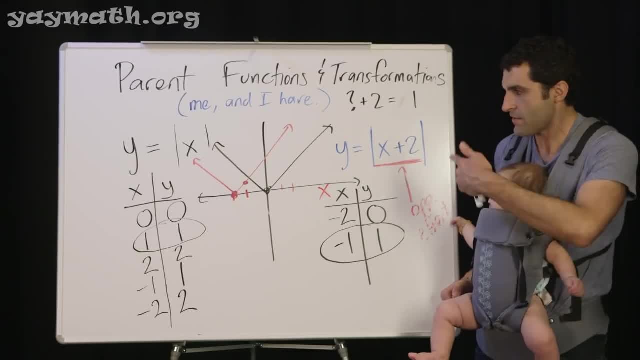 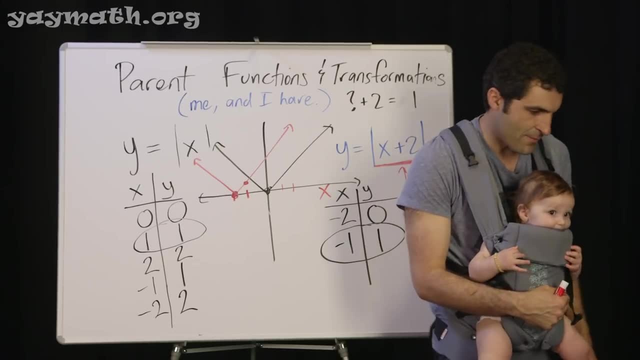 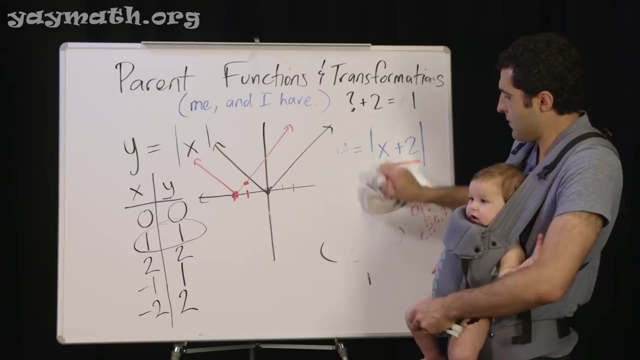 it as well. yeah, it's weird that it goes opposite when it's inside with X, but can you recover from that? okay, I'm glad, I'm glad. a few more transformations. let me get down to Buddha, Buddha, Buddha, baby, Buddha, Buddha, baby. I know, yeah, you feel the bicep. it's. 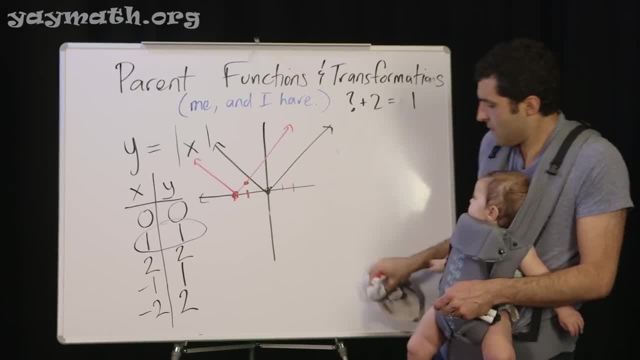 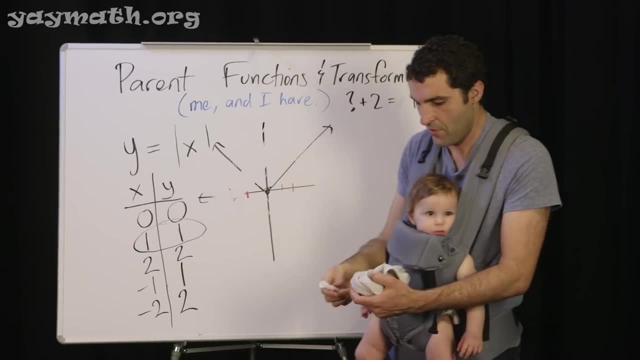 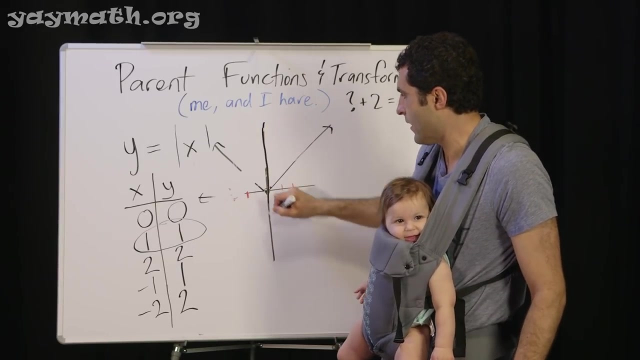 all because of you. it's all because of you. you gotta learn to walk one of these days. but you know I'm not rushing you. not rushing you. everyone's got to learn at their own pace. right now. focus, okay. so there you go. next transformation we did outside is up-down. 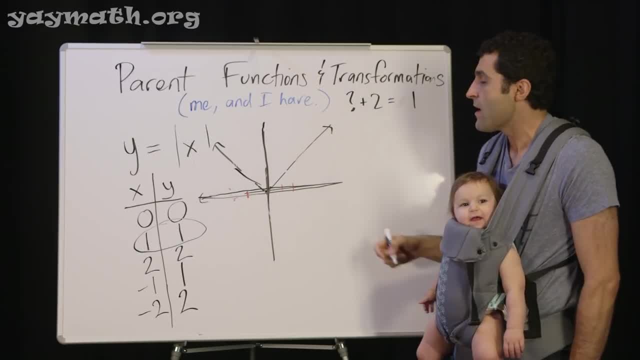 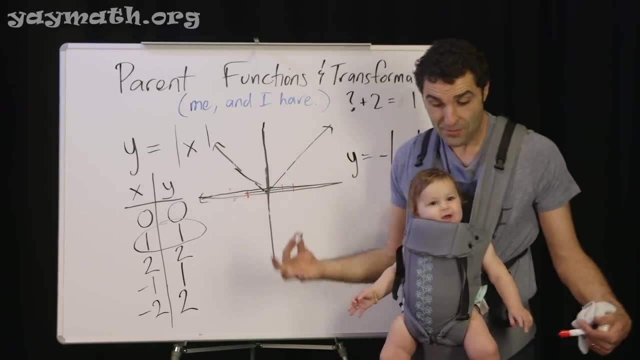 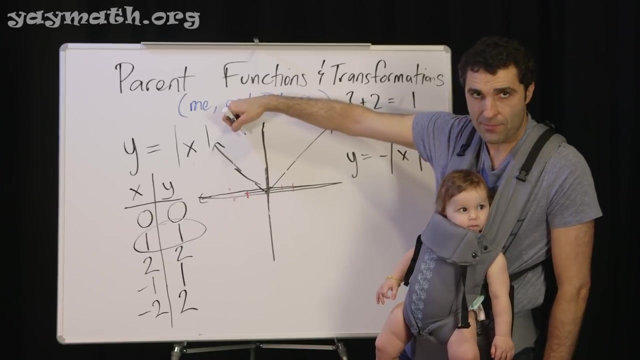 we did inside as left right, but opposite right. the next one has to do with making it negative. what's good about this is that these transformations apply to all parent functions, all parent functions. so if you go out here plus or minus something, it'll always go up-down. 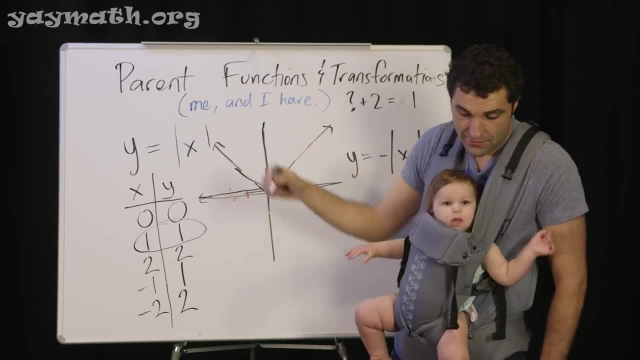 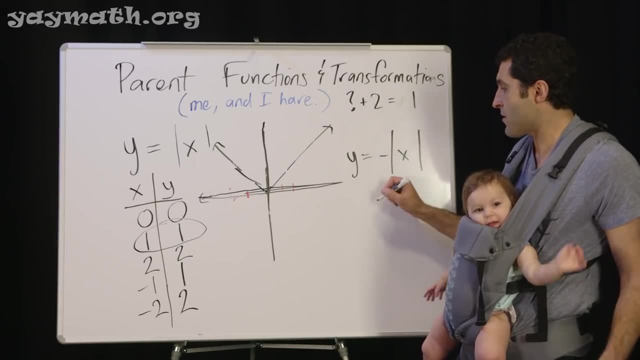 down. If you go inside left or right something, it'll always go left or right, but opposite. And now what does negative do? Best guess, Best guess, Yeah, think it through, Stretch it out. It's hard, It's hard to visualize, But once you put down the numbers, let's try. 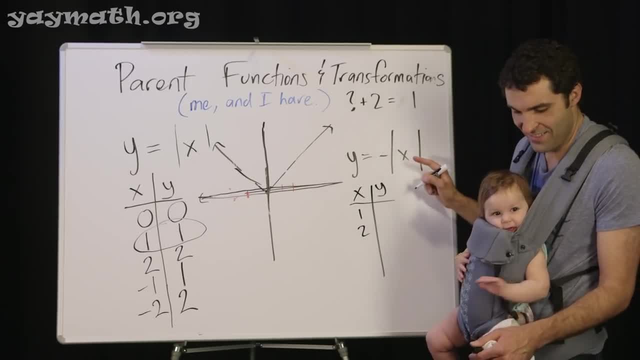 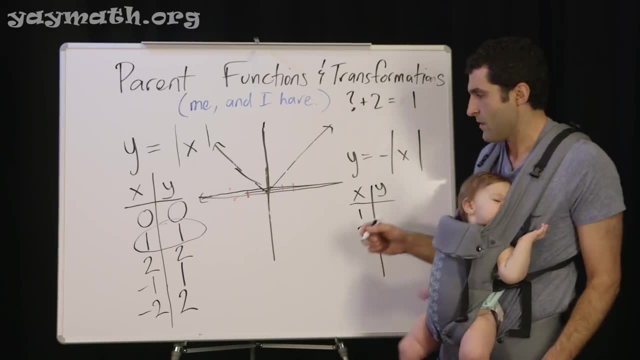 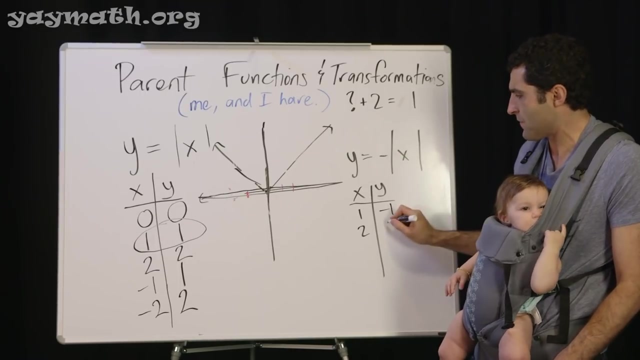 like one and two. I know I'm pleased. I'm pleased with how this is going And you feel surprisingly not heavy. So let's put down one here. That becomes negative one. If we put in two here, negative square root or absolute value of two is negative two, And you'll see. 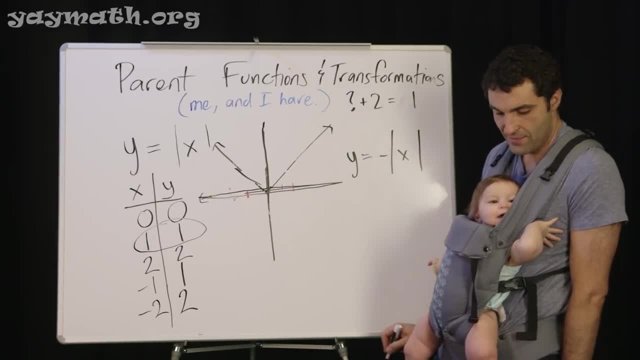 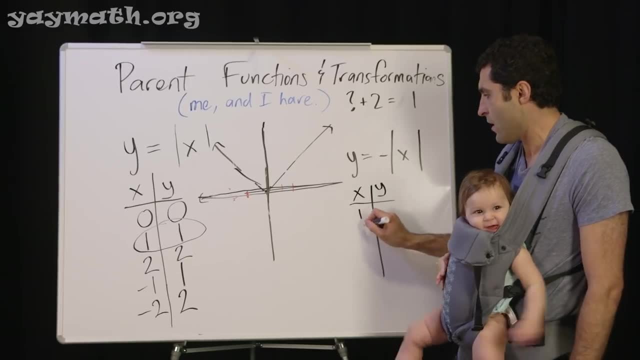 And now, what does negative do? Best guess, best guess, Yeah, think it through, stretch it out. It's hard, it's hard to visualize, But once you put down the numbers, let's try, like one and two. I know I'm pleased. 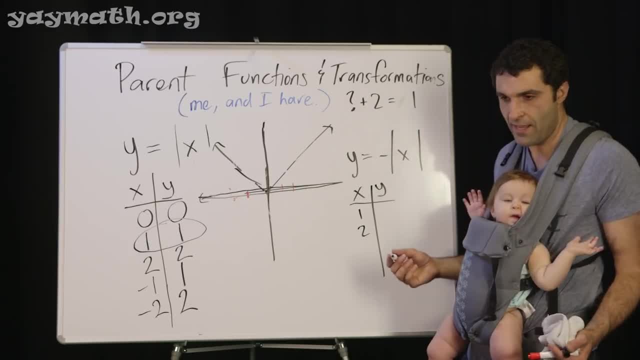 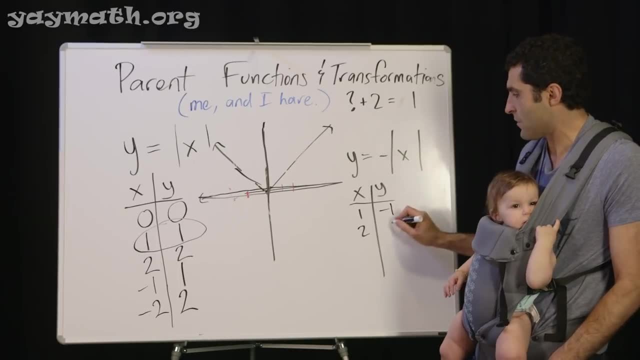 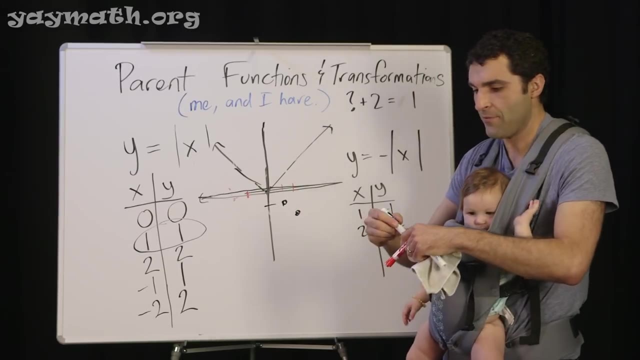 I'm pleased with how this is going And you feel surprisingly not heavy. So let's put down one here That becomes negative one. If we put in two here, negative square root or absolute value of two is negative two, And you'll see that you get this downy effect. 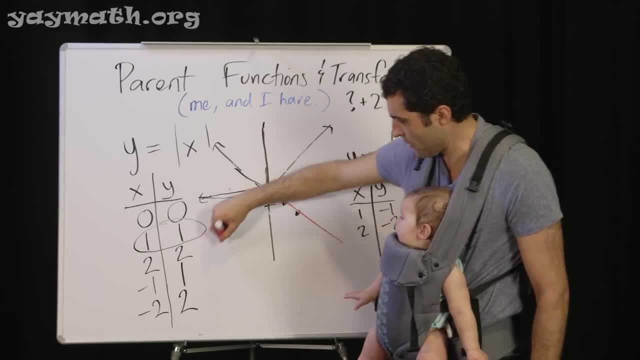 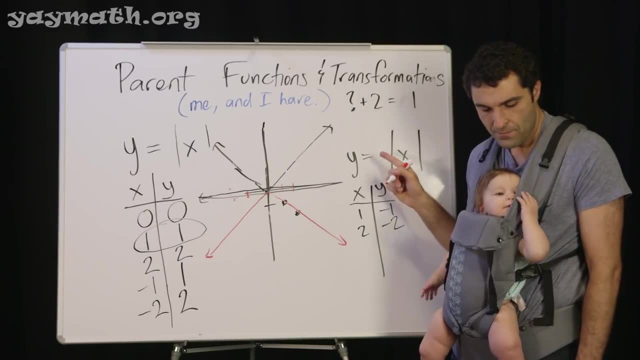 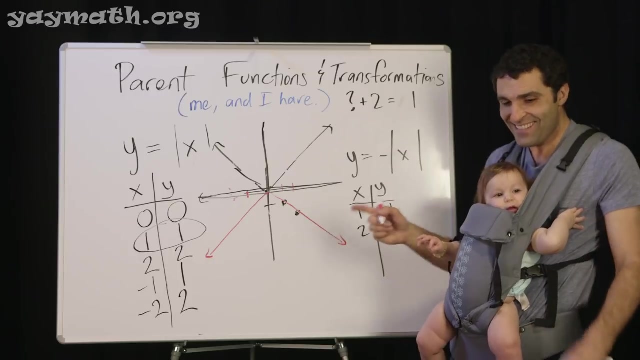 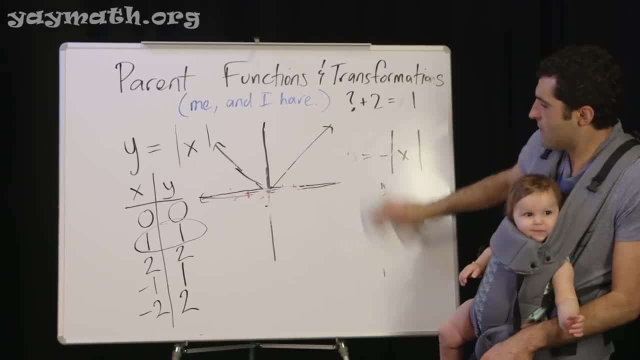 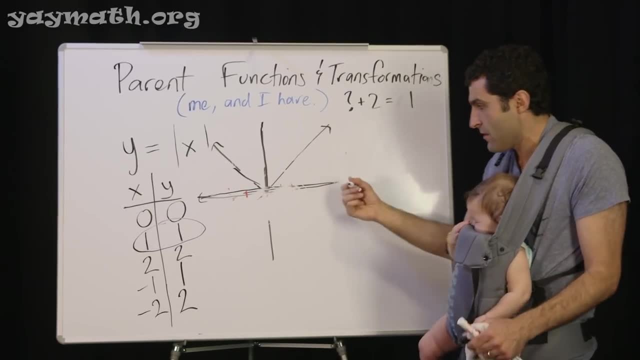 It flips down. It flips down. There you go. Good job. Kind of like my eye mask when I try to get some sleep at night. Yeah, I do wear an eye mask because I need the darkness. The eye mask flips down, just as like the negative. 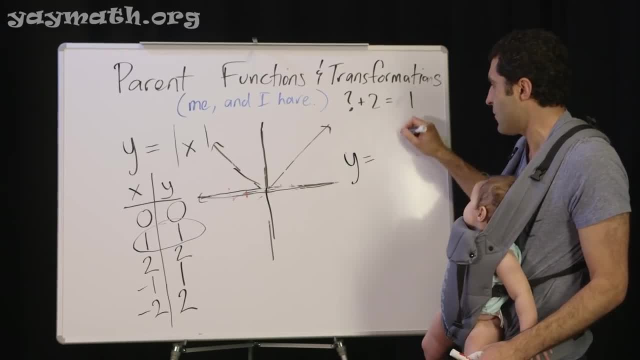 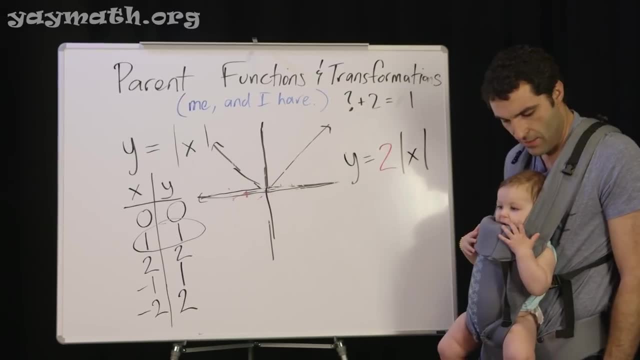 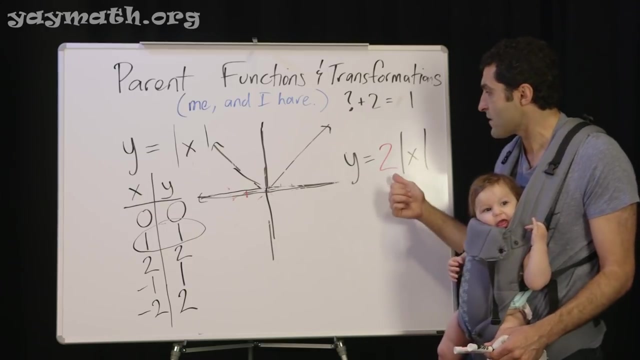 One more transformation to do, That is, if you put a coefficient or a number outside here. All right, You're ready to handle that one. Yeah, chew on that, Chew on that. It's actually very difficult to understand it. first, What does the two do? 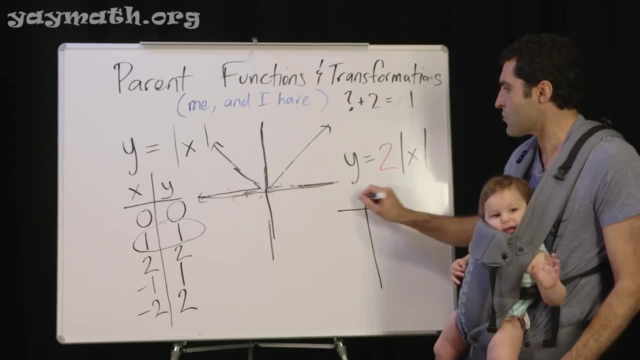 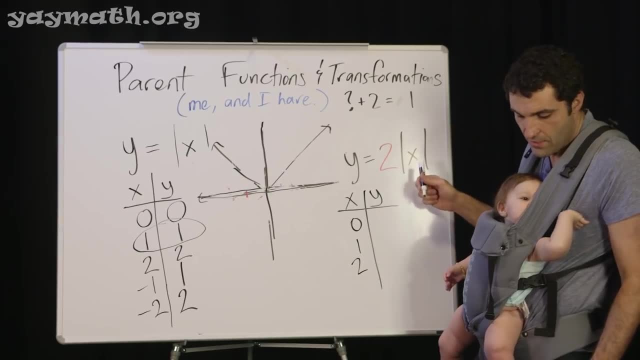 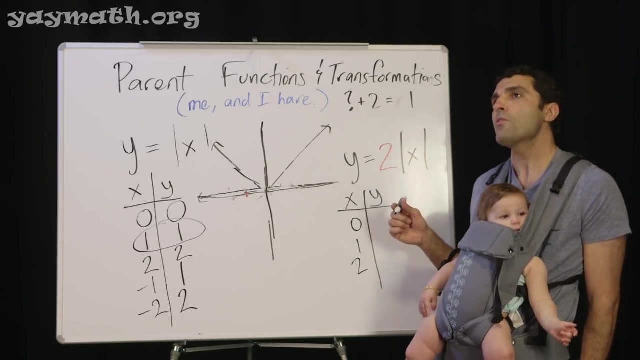 Let's find out. The two goes in front of the x. Zero, one, two. let's see what happens Two times the. I'm going to match your tone. You're right, it's important to have common energy. Two times the absolute value of zero is still zero. 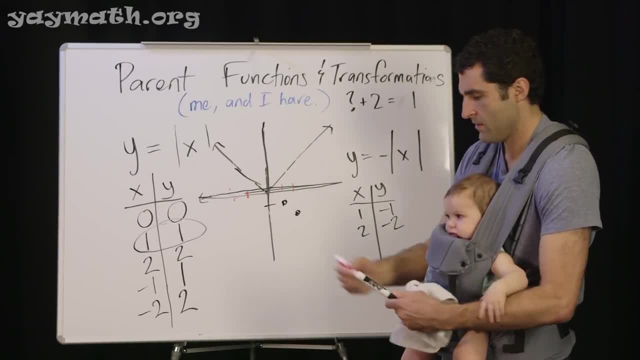 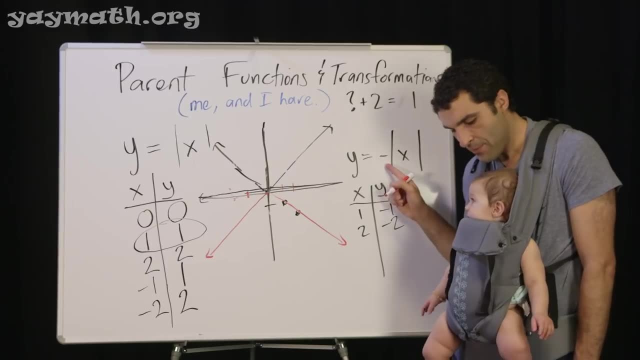 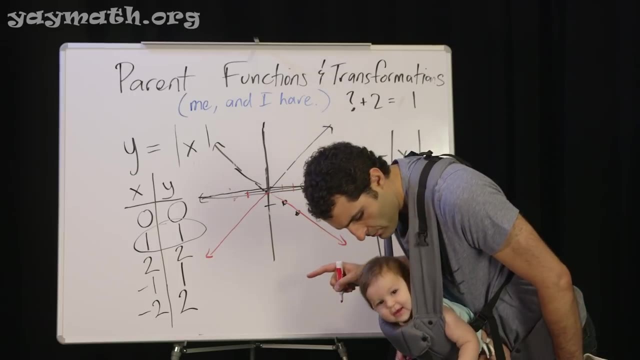 that you get this downy effect. See the downy Sort of like your fabric softener. There you go. So what happens when you put a negative outside? Where does it flip? Does it flip down? It does It flips down. 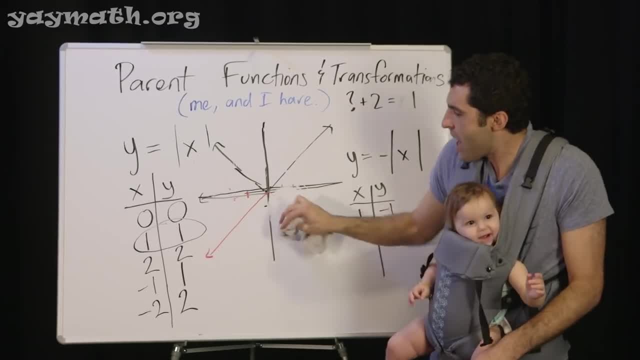 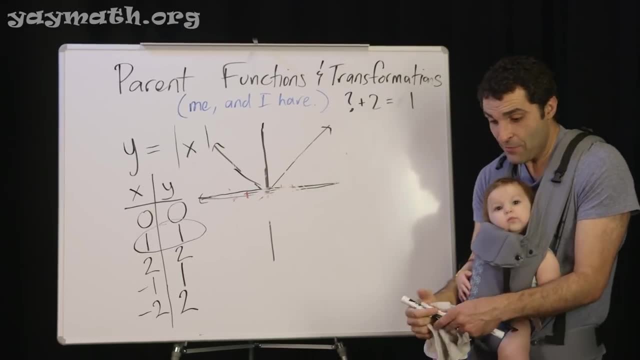 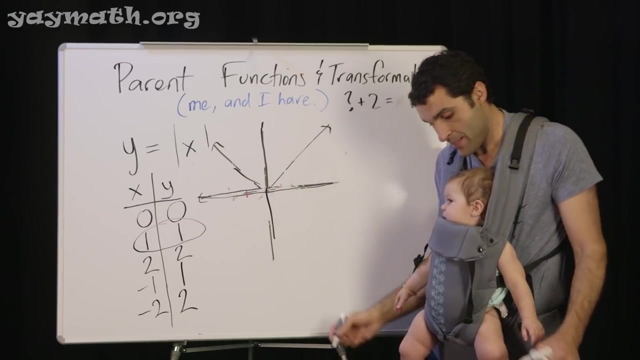 It flips down, It flips a down, It flips down. There you go, Good job. Kind of like my eye mask when I try to get some sleep at night. Yeah, I do wear an eye mask because I need the darkness. The eye mask flips down, just as like the negative. 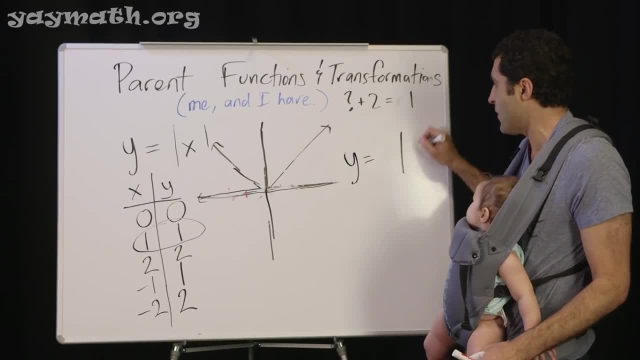 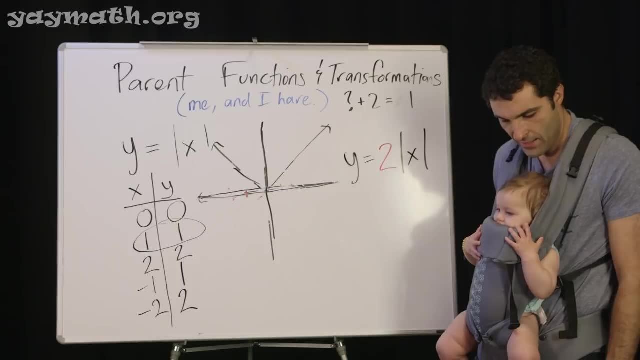 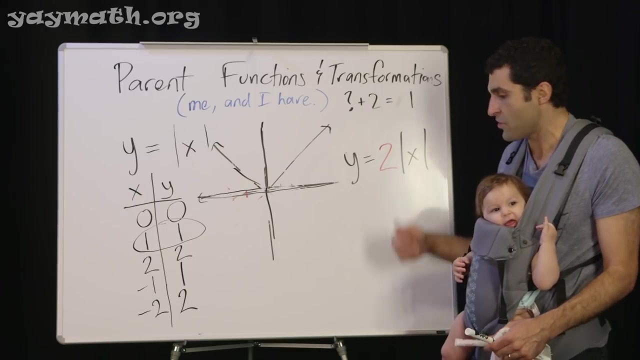 One more transformation to do. That is, if you put a coefficient or a number outside here. You ready to handle that one? Yeah, chew on that. It's actually very difficult to understand at first. What does the two do? Let's find. 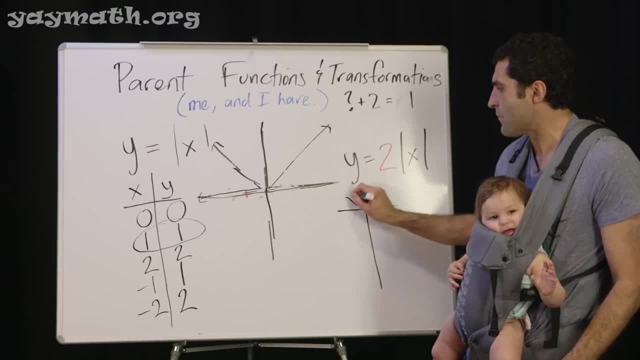 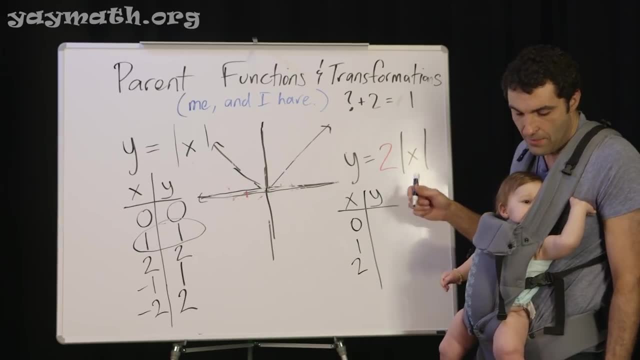 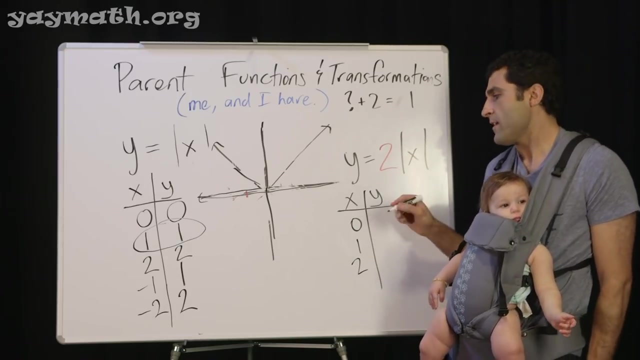 out. The two goes in front of the x. Zero one. two: Let's see what happens. Two times the – I'm going to match your tone. you're right, It's important to have common energy. Two times the absolute value of zero is still zero. Two. 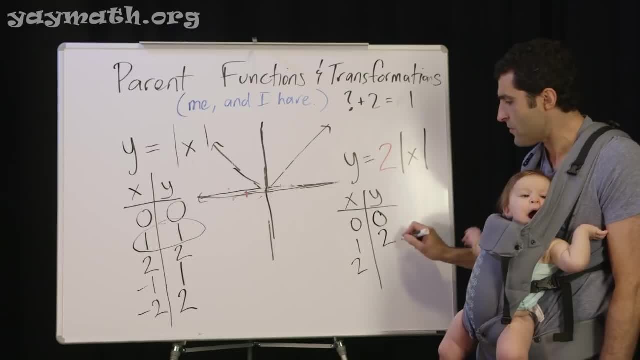 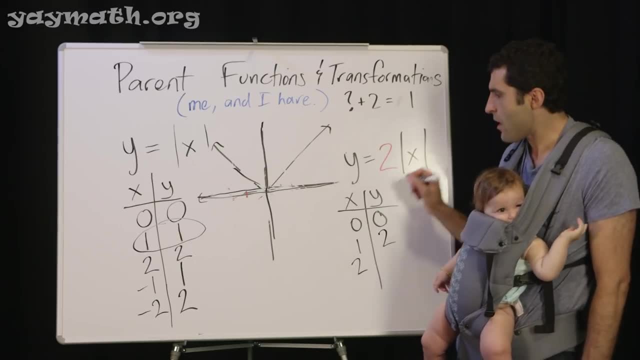 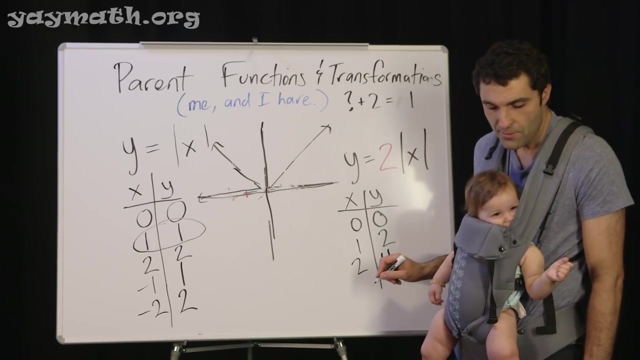 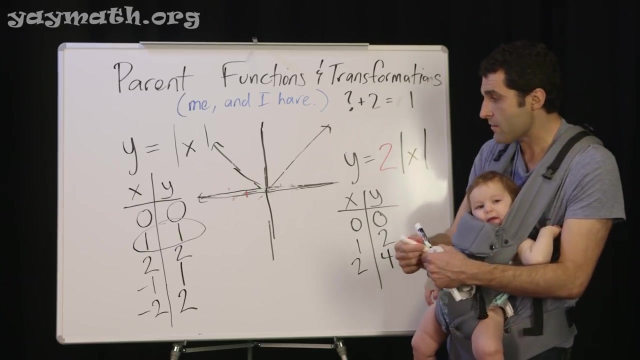 Two times the absolute value of one is two, And two times the absolute value of two becomes four. Are you asleep? I don't know if that's a compliment or not. Let's see what happens to the graph. little friend, Here we go: Zero, zero, One, two, Do you? 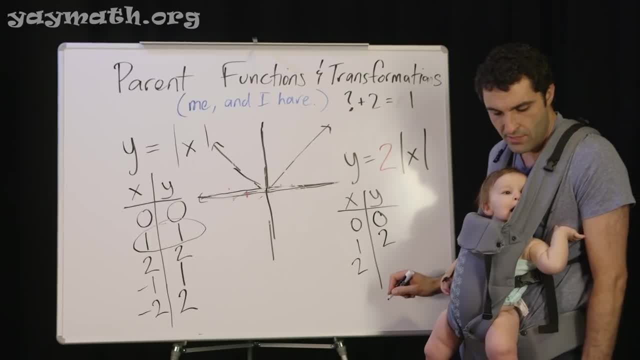 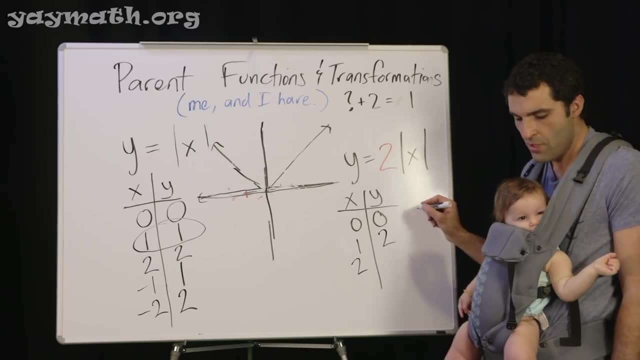 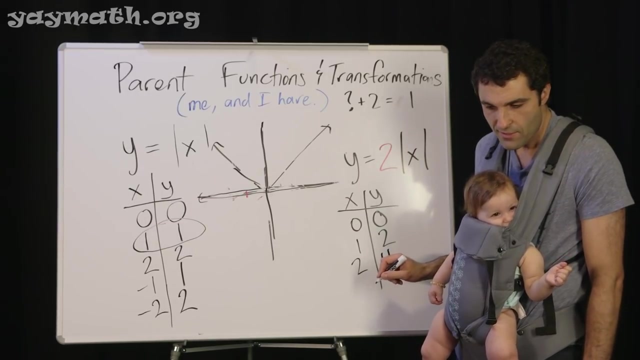 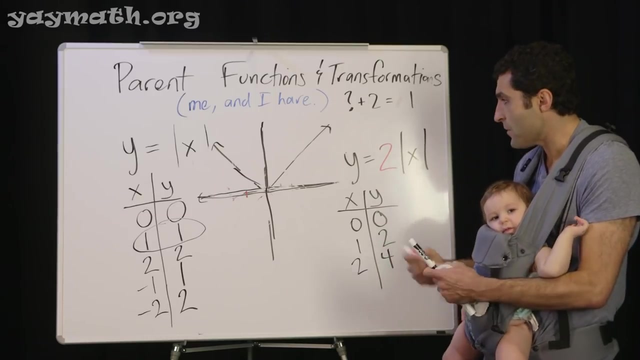 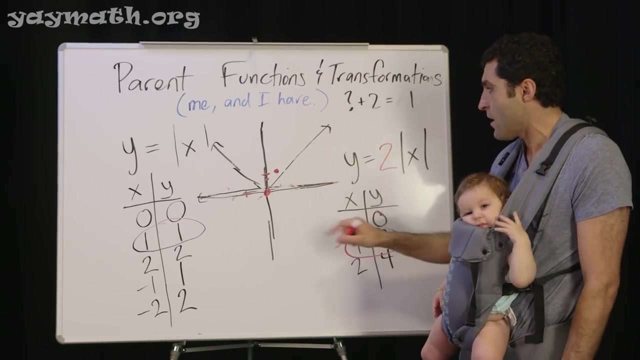 the absolute value of one is two, and two times the absolute value of two becomes four. are you asleep? i don't know if that's a compliment or not. uh, let's see what happens to the graph. little friend, here we go: zero, zero, one, two. do you see this? uh, what's happening to the graph? instead of one, one, 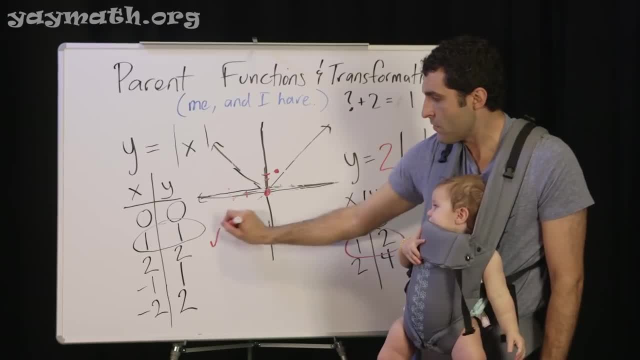 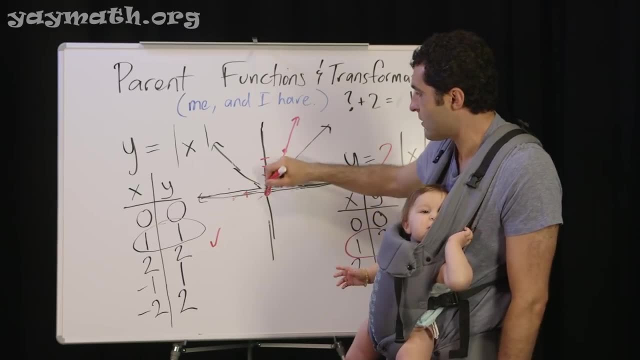 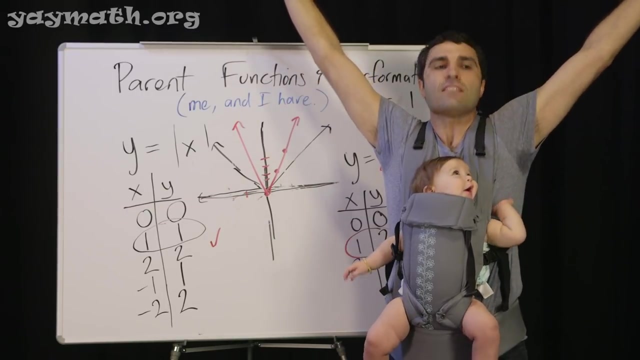 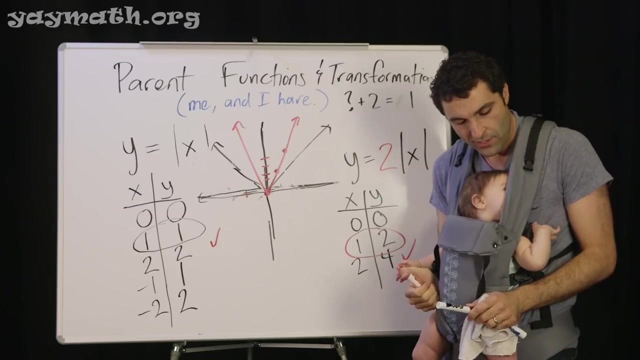 we have one, two instead of two, two, we have two, four. oh my goodness, oh my goodness. it looks like the graph is stretched vertically. it's stretched vertically. oh yeah, you're tired. get like that after a long day too. you are such a warrior. so if there's a positive two, here it. 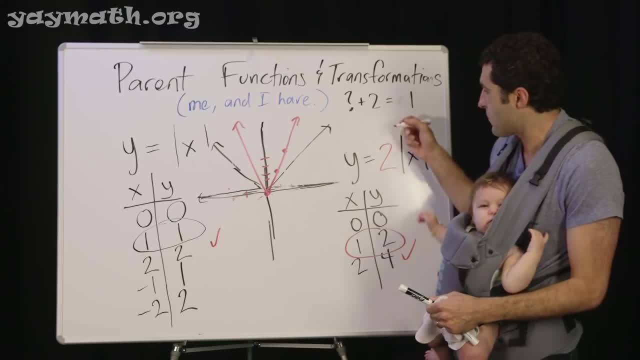 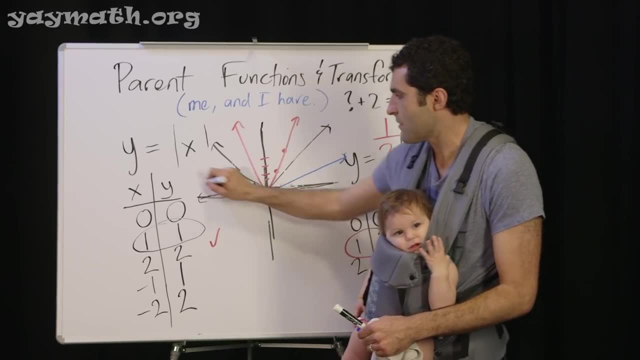 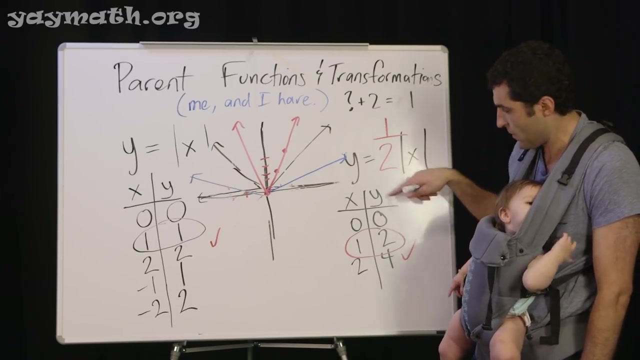 stretches vertically high, and if it was one half, it would actually be stretched out like this. does that make sense? now y is flattening, as opposed to y here getting big. here y is getting really big and here y is flattening out. it's just getting smaller and smaller. does that make sense? 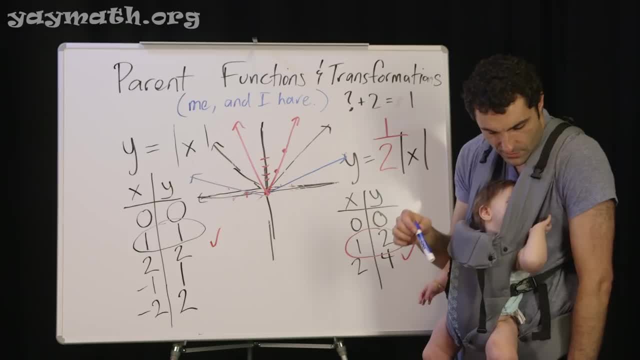 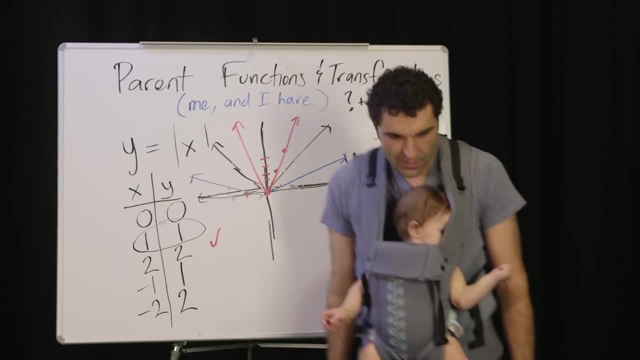 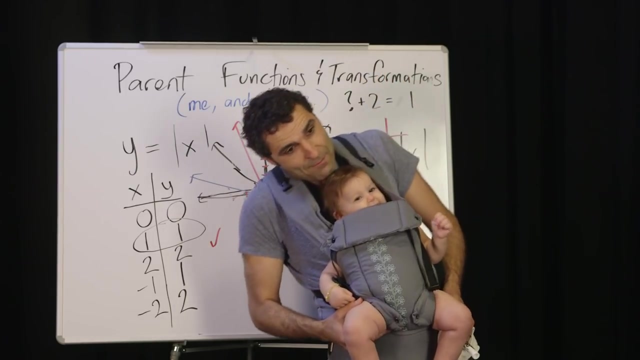 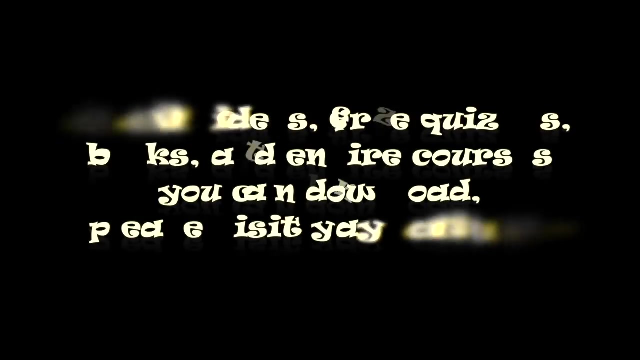 you want to take a turn. you're shy, how are you feeling? okay, we're gonna say bye now. we're gonna say bye. we're gonna say bye, yay, all right, that's good enough for me. bye you.